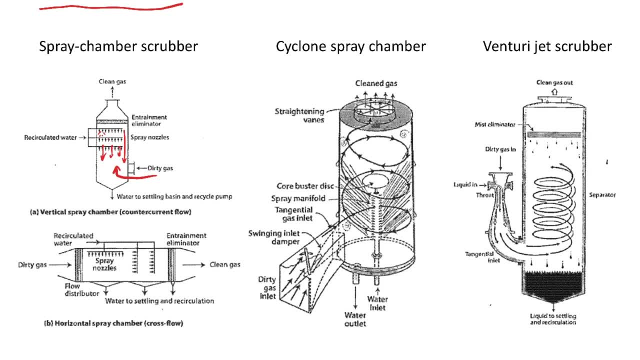 collide with the smaller particles and then attach them and then basically clean them up right and then, because of the higher gravity of the water droplets, it's just going to settle down. So I would say it's a combination mechanism of the gravitational settling and cyclone. 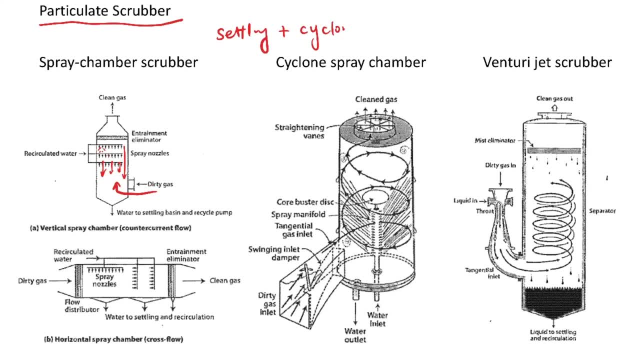 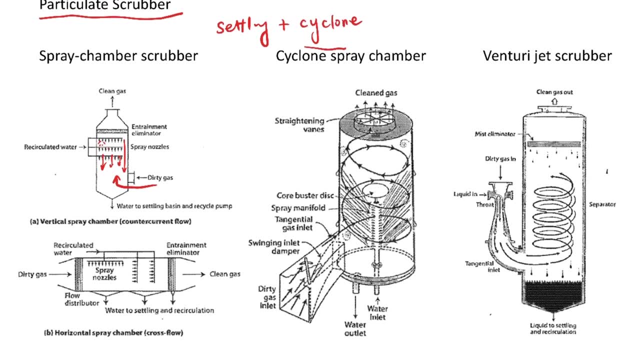 Okay, the cyclone uses the uses inertia, right, for example, this type of scrubber here. so we're introducing the air in this rotation or swirl pattern, right, and then the larger particles will just get removed from the stream. right, we have a higher inertia and then at the same time, we 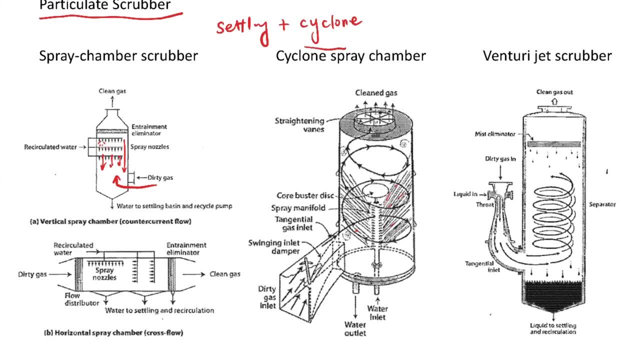 spray water droplets to the wall. So in this way the particle basically will become larger. right, due to the water, are colliding with a particle and because of the larger size they're going to have a higher inertia so we can more efficiently remove these particles. but still the particle scrubber has the problem of 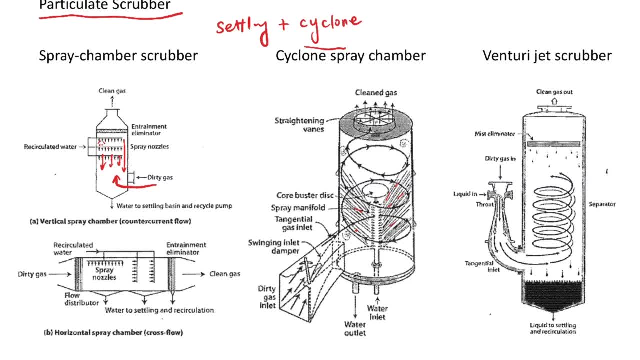 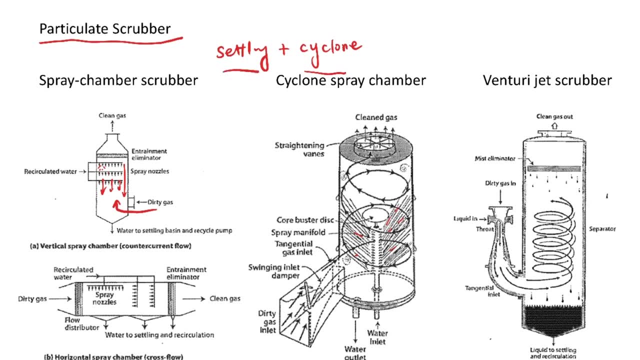 low efficiency for very small particles. so, because it's still utilizing the settling and the cyclone right, we know that these two are not very efficient for very small particles. so to remove those very small particles, we still need to refer to the esp or the backhouse filter right. 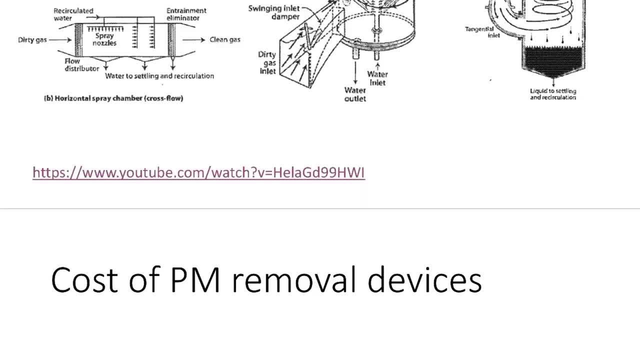 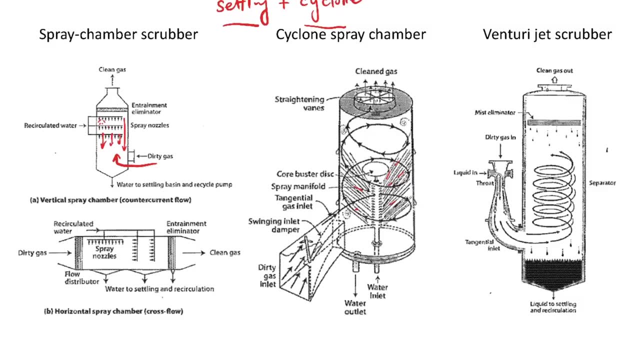 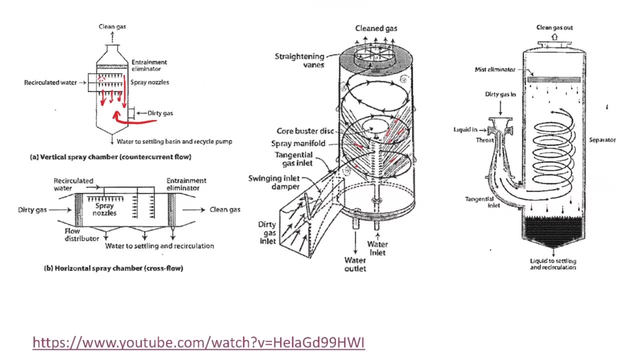 in terms of the efficiency of this, of this particle scrubber, there's a set of equation that we can use. so, basically, if we want to calculate the efficiency of the device, we need to first know what is the penetration right? so so the penetration is basically one. 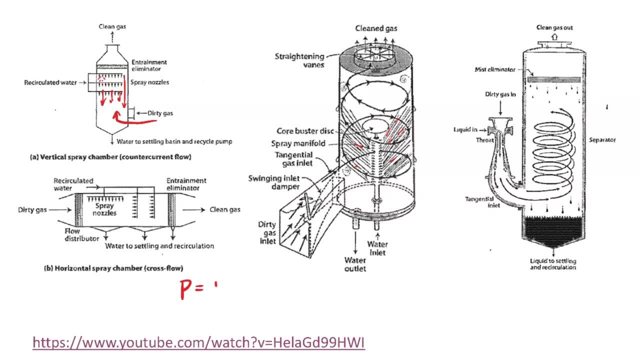 minus the efficiency of the device, right, so the penetration is basically one minus the efficiency. so this is a fraction of particle that can exit through the particle scrubber and that follows the equation of exponential minus a, d, vt, e to d divided by q, g. okay, so it is a quite complicated. 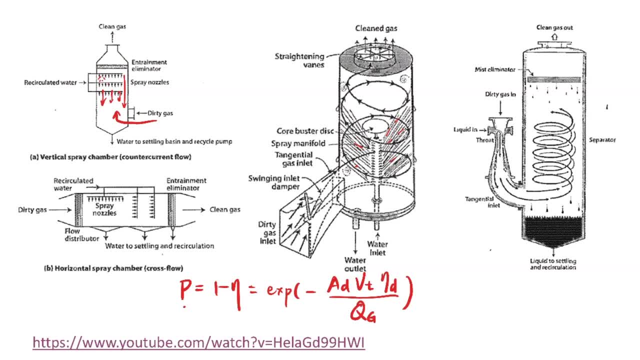 equation here. so, but if you think about the mechanism for removing these particles, these parameter parameters actually make sense. so let's say first a d here. let me just label this out. so a d here is the cross-section area of all droplets. so what this means is that if you consider the water droplets being sprayed down, 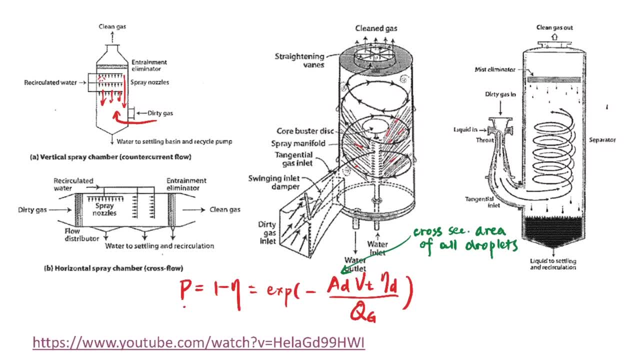 and then if we just take a cross-section, so what is the area of all the droplets in there, right? and then let's think of two extremes. so let's say: if there's no water? so if there's no water, then that basically means that a d is equal to zero, right? if a d is equal to 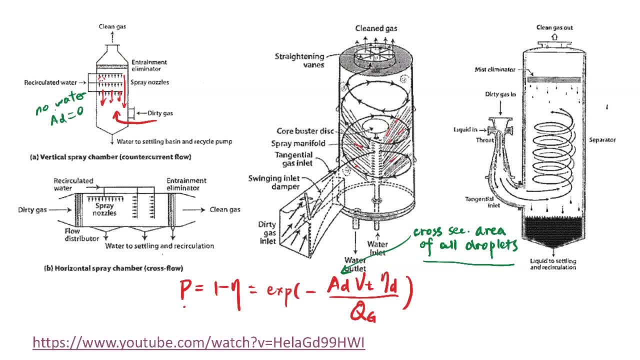 zero, then if you plug that in this term is zero, right equals to one, which means that all of the particles will penetrate through this particle scrubber right. and let's say, if a, d goes to infinity, so it might be too extreme here. so basically, if the add is infinity, then this is just like. 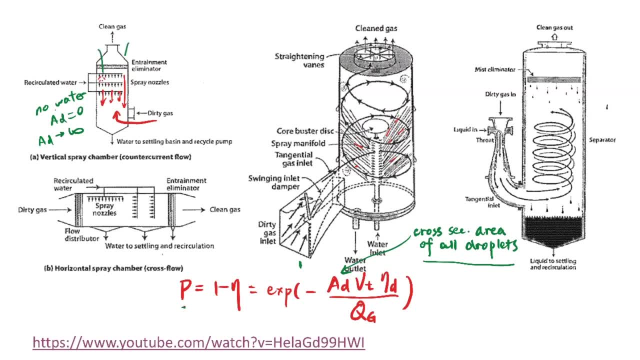 a faucet, right, so we're just flushing water through, so no particles will penetrate. if no particle penetrate, then basically this penetration should be zero. right, that works for here too, because ad goes to infinity. this whole term goes to negative infinity, which is equal to zero, and then the efficiency will be 100. right, so this term makes sense. and then vt. here is the terminal. 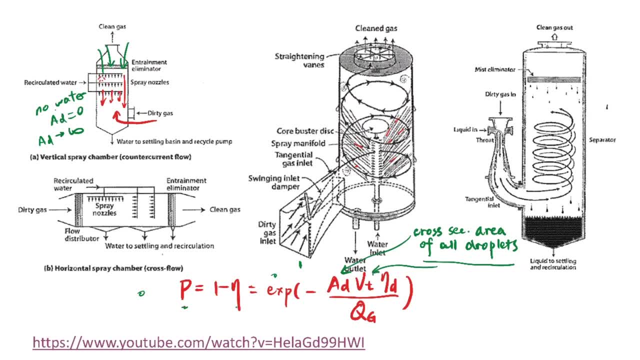 settling velocity of droplets. okay, so also, let's say, if the settling velocity of the droplet is very low, then that basically means that the it's going to take a very long time for the droplet to settle down to the to the bottom right and also, typically, if it has, if the water droplet has a 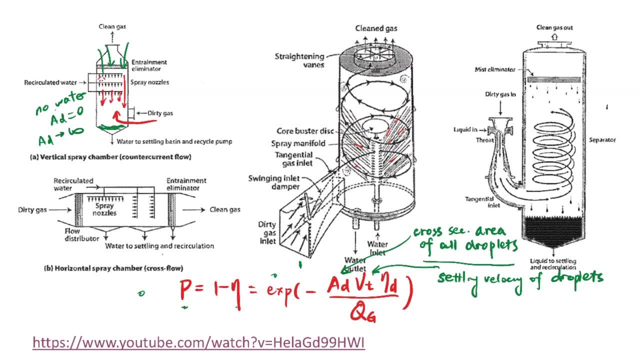 lower settling velocity means that the size is smaller. Actually, we're introducing more PM into the system, which is more difficult to remove. That's why the VT will affect the system. and then this eta d here is the efficiency of a single droplet in particle removal. 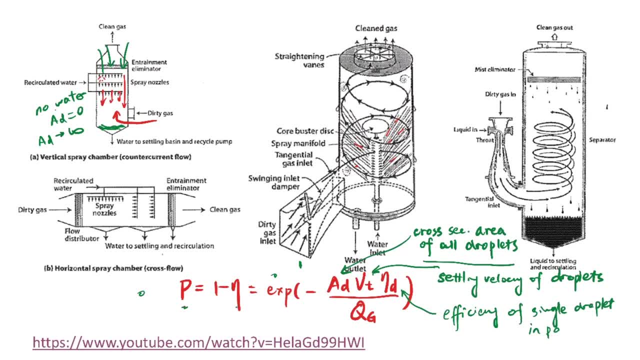 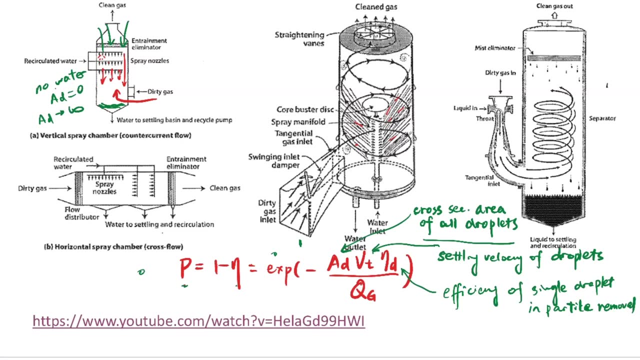 So we need to consider the detailed physics in this particle removing process. So basically, because finally it's just the interaction between a single droplet and some tiny particles surrounding it, So we had to somehow calculate this single efficiency here and plug that into the 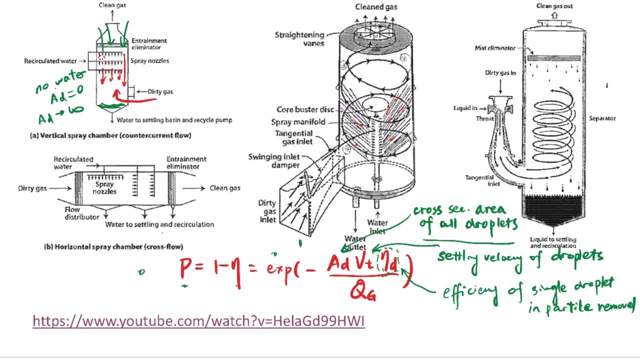 system. So let's say, if this single droplet is very efficient, then that means the particle removal will be more efficient. So we need to consider the penetration will become lower. If this single droplet is not efficient at all, then this eta d will become zero and then the penetration will be 100%. 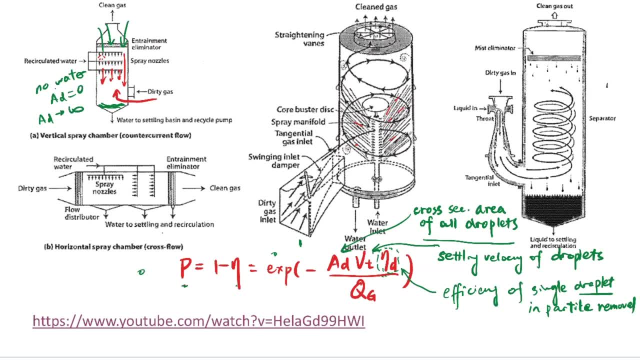 So this factor also affects the efficiency. And finally, the QG is the total flow rate of water. It's a total flow rate of gas. It has the G here, the total flow rate of gas. So similarly, let's say, if the flow rate of gas is very high, then it means that 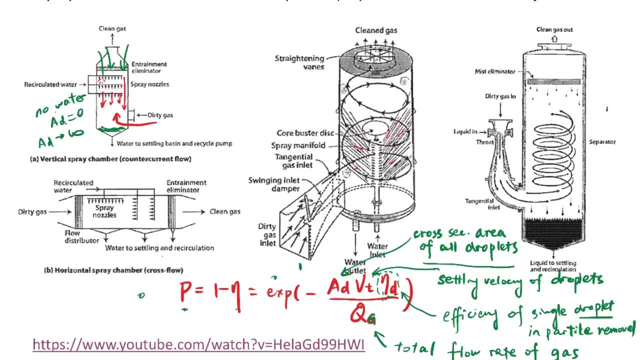 this process will become less efficient. Let's say, QG become higher and this whole term, this fraction, becomes lower and then, because it has the negative sign, this whole term in the exponential become higher. So basically it means that if the QG becomes higher, the penetration becomes higher, The system becomes more efficient. 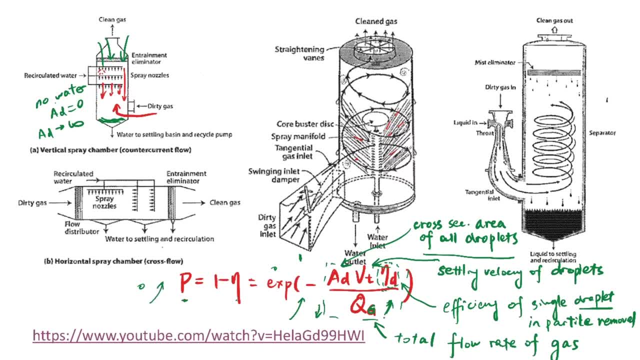 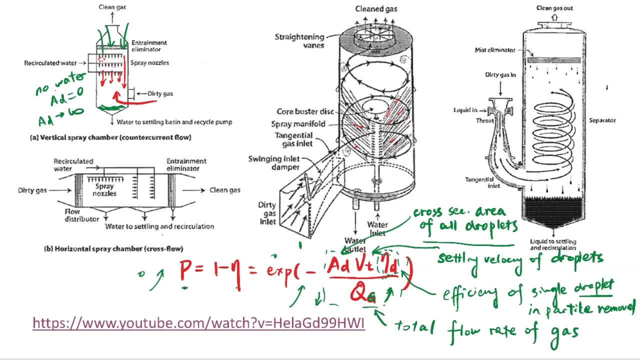 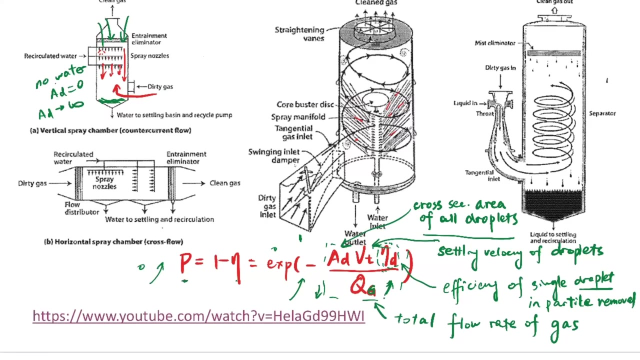 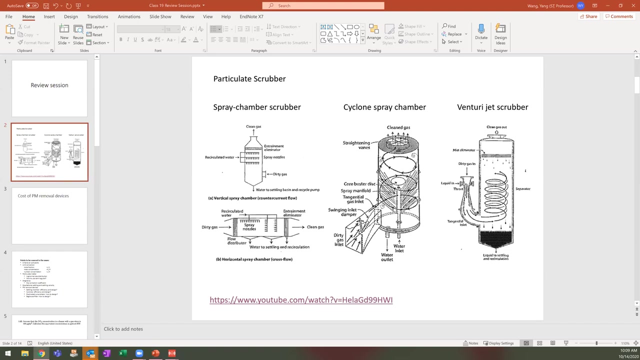 So basically all of these parameters make sense in this equation here, And this is kind of like a equation that's based on the experiences of engineering operation. So here I also have a short video of the particle scrubber. A packed bed scrubber, also called packed tower scrubber, is designed to remove. 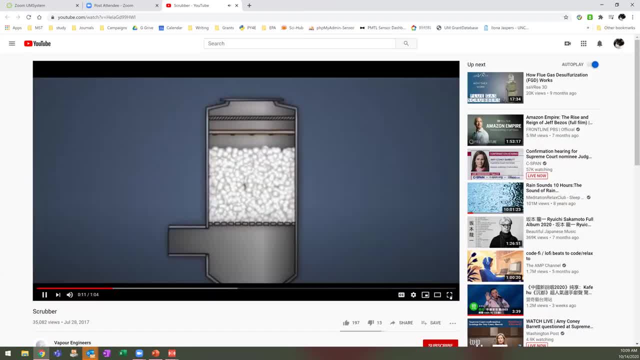 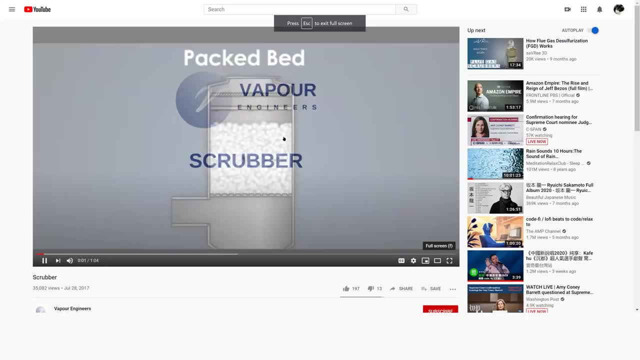 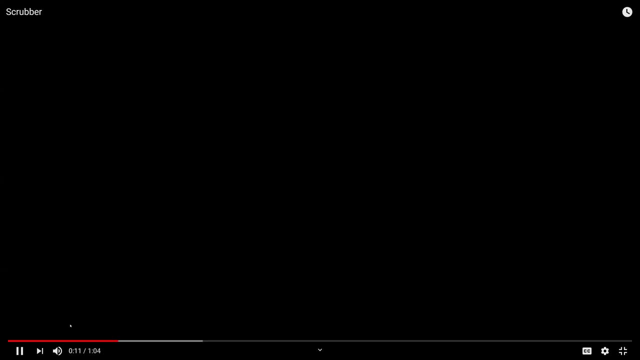 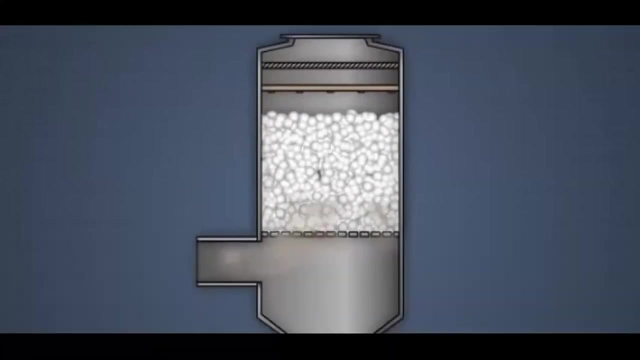 both particulate matter. A packed bed scrubber, also called packed tower scrubber, is designed to remove both particulate matter as well as gaseous pollutants. The contaminated gas stream is fed into the tower. Inside the tower is a bed of special packing material: Nozzles spray. 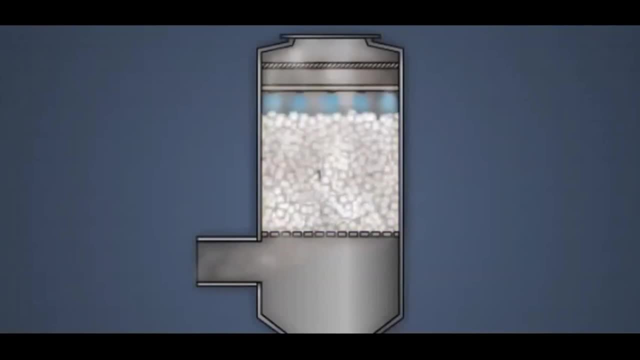 scrubbing liquid on top of the packing material and the liquid works its way down the tower. As the gas passes up through the packing material, the particulate and gas molecules come in contact with the film of scrubbing liquid on the packing. The particulate and gas molecules come in contact with the film of scrubbing liquid on the packing. 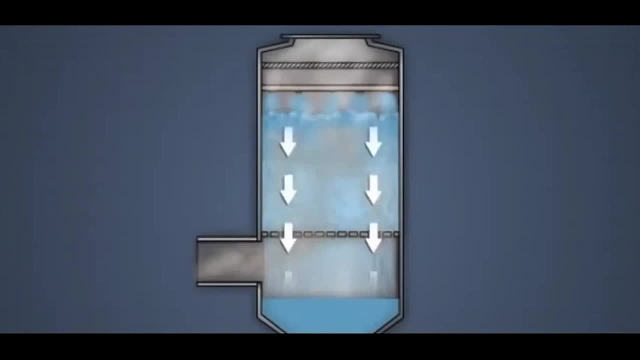 Contaminated liquid drains down through the packing material, past a packing support and out through the bottom of the tower. The gas stream flows out through the top of the packing material, past the nozzles and through a mist eliminator before exiting the tower. 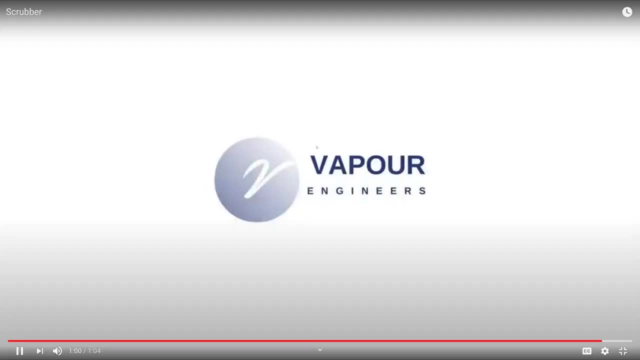 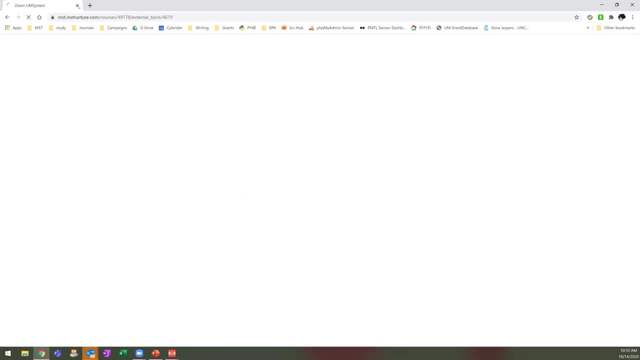 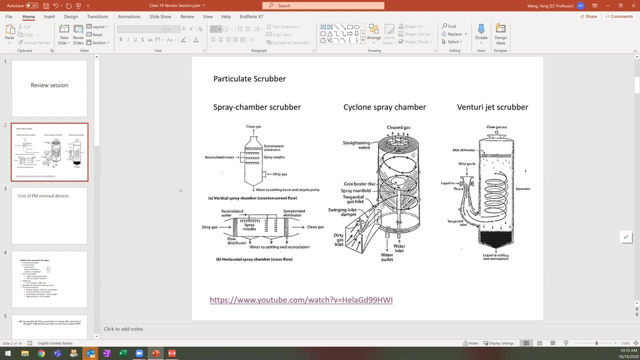 Okay, so this is one type of the scrubber. So the scrubber means basically the cleaner, because scrub means clean something up, right, So scrubber means cleaner. So the advantage for the scrubber is that it's not only cleaning the particles. 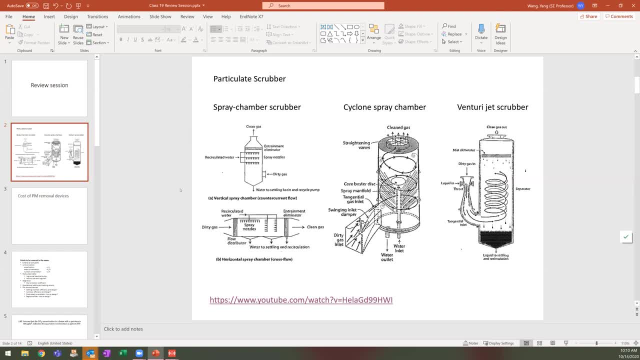 The design of the scrubber is mainly targeted at the gaseous pollutants, for example the sulfur dioxide, nitrogen dioxide. So while it can absorb or remove those gaseous pollutants, it can also remove the gaseous pollutants. So while it can absorb or remove these particles here, 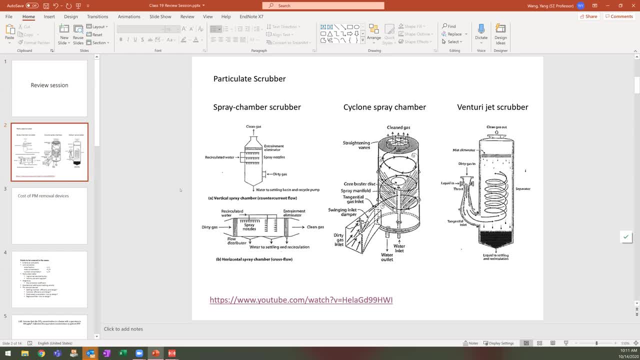 So that's why we also want to introduce this particle scrubber in the PM removal devices. So we will learn more about the scrubber system when we talk about the control of the sulfur dioxide, Because we know that coal-fired power plants- they just generate millions of tons of sulfur dioxide every year, right? 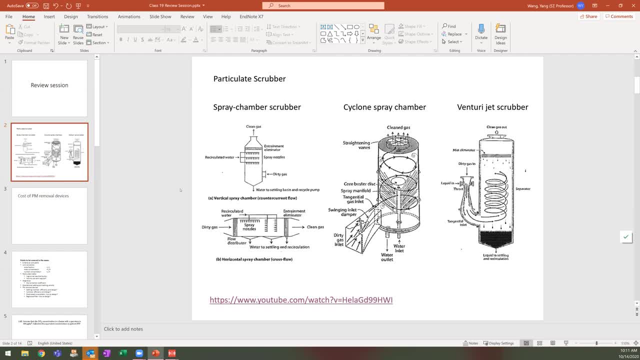 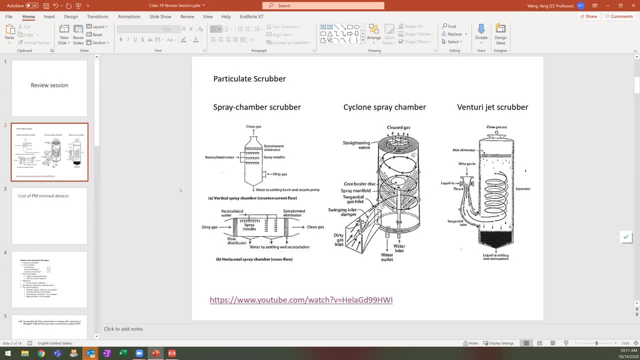 And the system that we use is actually the scrubber right. So this is the final PM removal device that we want to learn about. There's not a lot of design systems, design problems associated with this system. So, finally, we need to talk about the cost of the PM removal device. 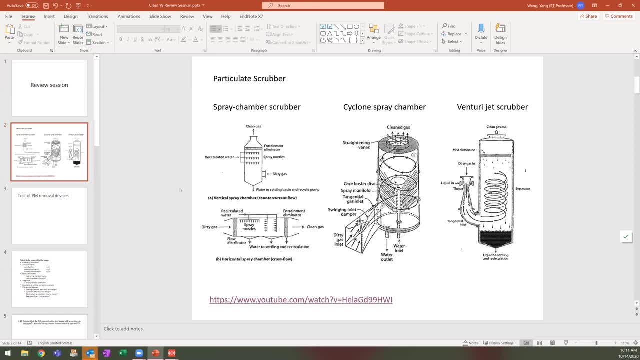 So if you read the textbook, you will see that in the textbook for each chapter where it talks about certain components. So if you read the textbook, you will see that in the textbook for each chapter where it talks about certain components. certain PM removal device. 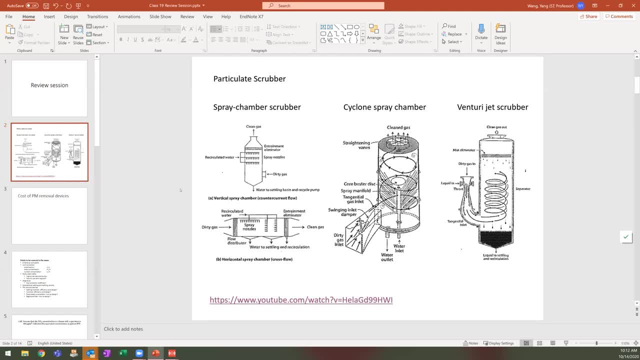 At the end it also describes the cost right. So the cost will include both the capital cost or capital investment, which is the cost for building construction, constructing this PM removal device, And also you have the operation or the operating cost. 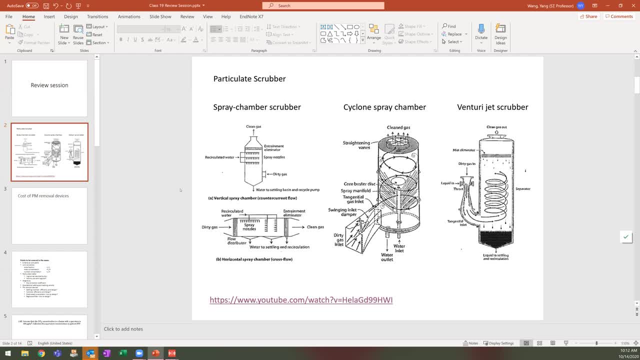 So the operating cost first of all is the cost of the PM removal device, And the operating cost of the PM removal device is the cost of the PM removal device, for example, the ESP electrostatic precipitator. we need to connect it to a certain high voltage right. 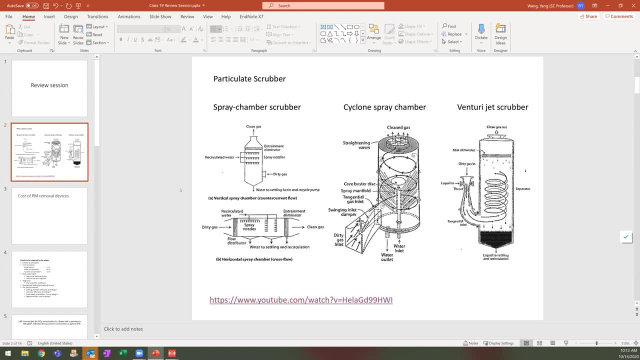 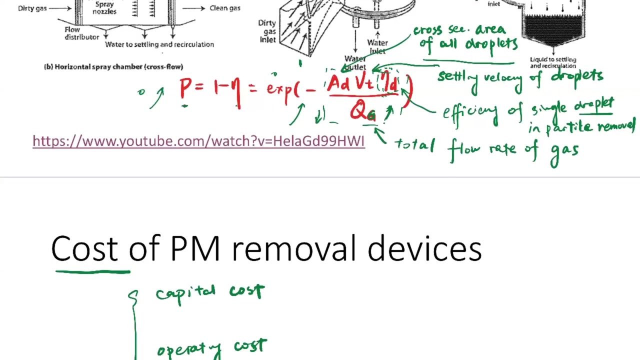 So it's going to use some power And also for any-. May you please share your screen please? Oh yeah, that's right, Let's see. Yeah, thanks, I just realized this. I just wrote two lines here. Maybe we can start up. 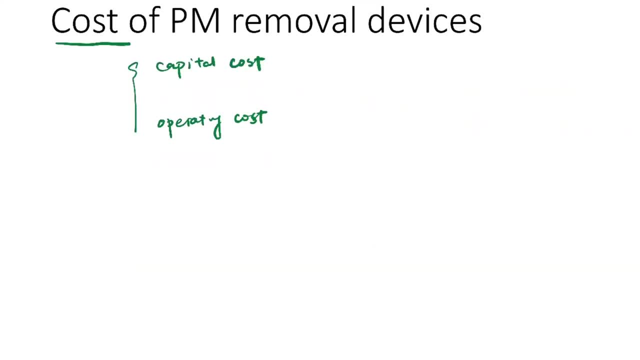 So we haven't discussed the cost of the PM remote devices yet. So, as I have introduced, the cost will mainly include the capital cost, which is for constructing the system, and also the operating cost, As we have introduced the ESP and back-off filter. 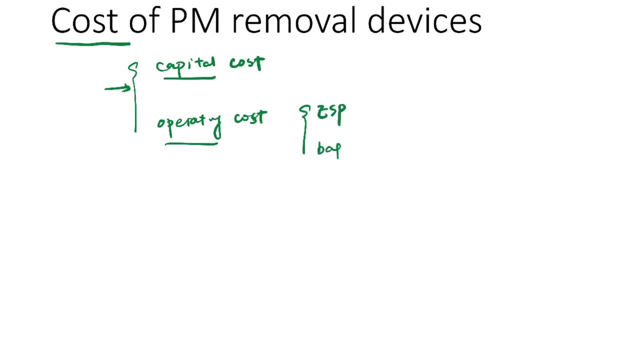 it's going to require a pretty high operating cost, right, Because we need to connect it to a certain high voltage power supply And also for the back-off, we need to replace the backs. quite often We need to shut off the compartment off for some time. 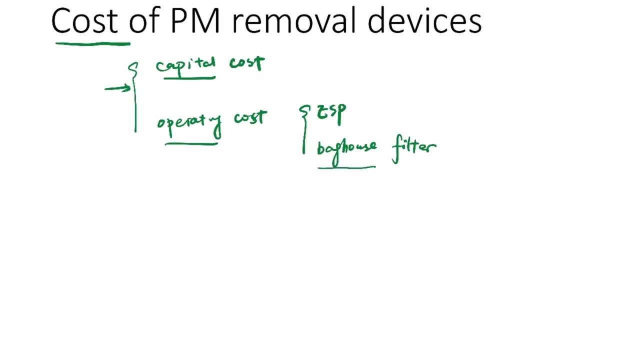 and then connect it back online. So these systems are going to cost quite a lot of operating costs. But for the power supply, we need to replace the back-off filter. So we need to replace the back-off filter. So we need to replace the back-off filter. 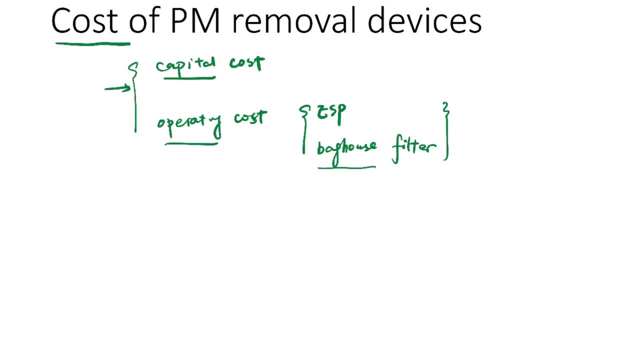 So we need to replace the back-off filter, But, for example, for the cyclones. so what we mentioned is that cyclone is basically just a metal case, right? So once it's set up there, it doesn't need a lot of maintenance. 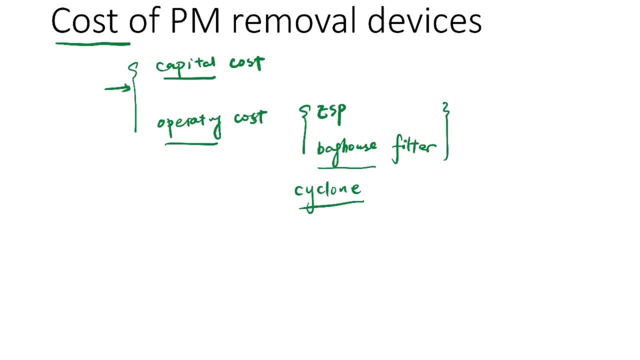 We're just passing through the flue gas, through the system. So there are definitely some differences for each type of the PM remote device. And in your project, team project, you're going to go through the details, You're going to go through the cost analysis. right, 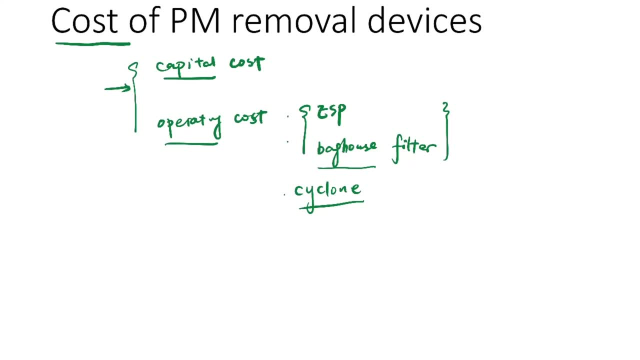 So what is the cost for building up such a PM remote device? And for this class we're just going to talk about very basics in this cost analysis. So typically the cost of these PM remote device, let's say we're going to use the equation: 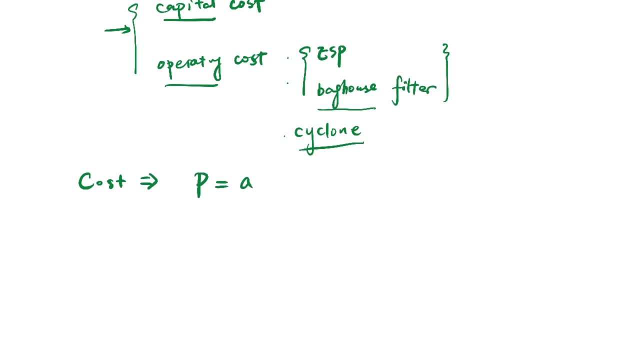 P equal to A, X to the power of B plus C. okay, Let's say we're going to use the equation P equal to A, X to the power of B plus C. okay, So the X here is related to the operating parameter of the device. 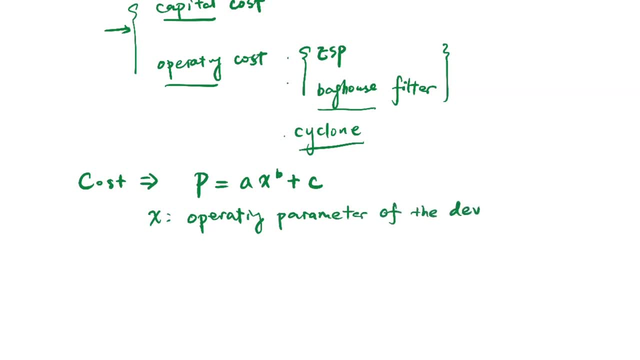 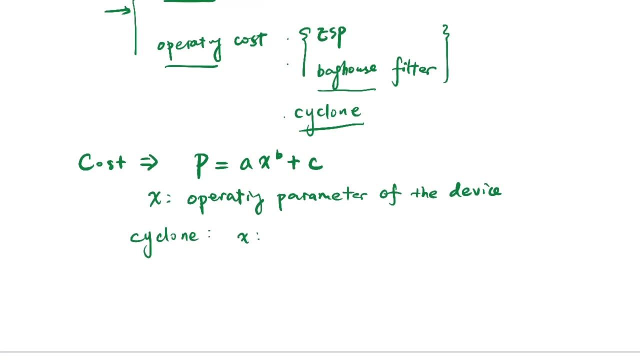 So, for example, if we're talking about the cyclone right, so the X will be the cyclone inlet area. As for case B- putting in some of these different camer providing support, right X will be the most descent фильм. 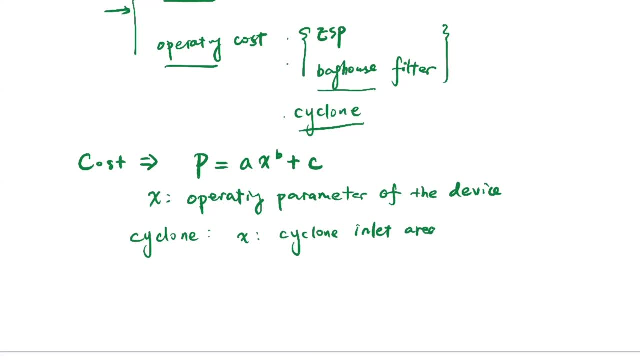 okay, so it might sound quite arbitrary here, So a minute sounds quite Marie out, But this is what people find out basically, like building different types of the cycles. what they find out is that actually the cost associated with the cyclone can somehow scale. 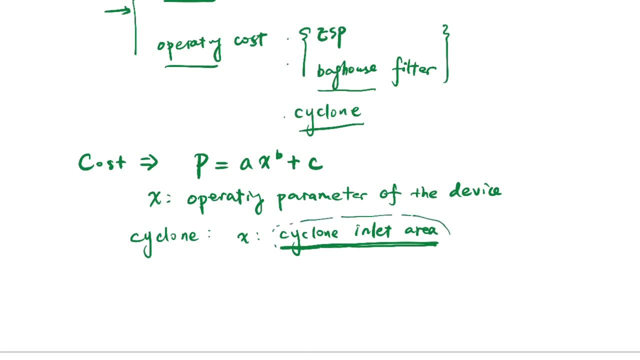 is the inlet area of the cycle. So because the inlet area determines the geometry right- And we mentioned that, for example the cyclones- it has a set of geometry, let's say the, the lapel type right. once you know the diameter, you should be able to calculate all the different dimensions. so this x here is related to the. 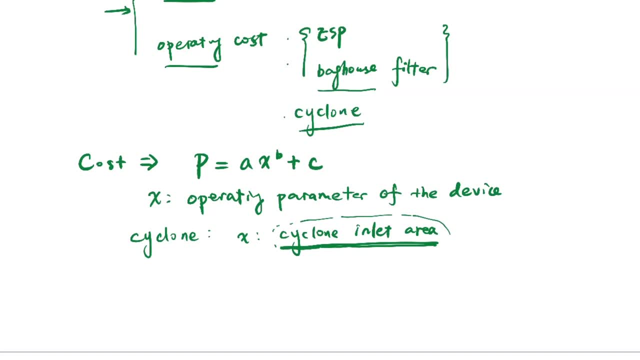 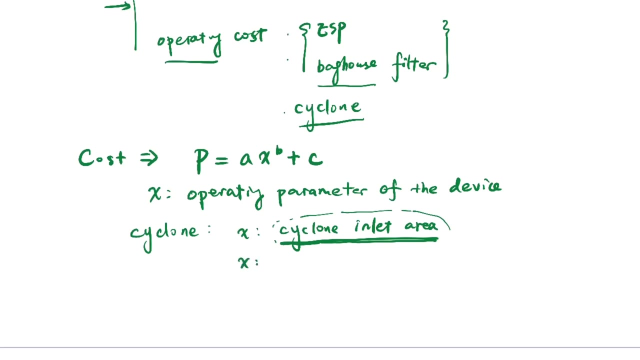 to the inlet area of the system. yeah, see someone still in the waiting room. probably have been there, has been there for quite a long time. so, and for the and for the esp, the x is related to the plate area or this total plate area. okay, this kind of makes sense, because the the cost of the esp is mainly, i would say. 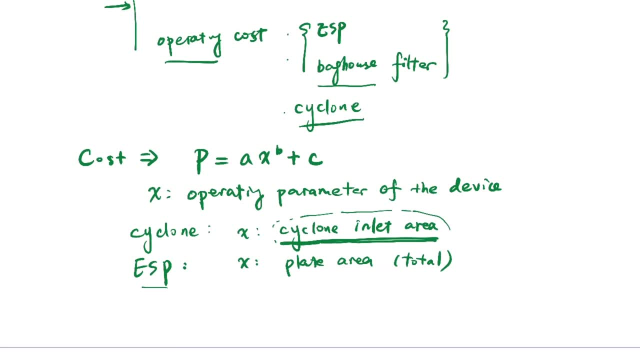 largely determined by how much plate- even how many plates- we're going to use, right? so that's related to the total plate area. and for the back house, this x is related to the cloth area. and finally, for the scrubber, this x is related to the gas flow rate. 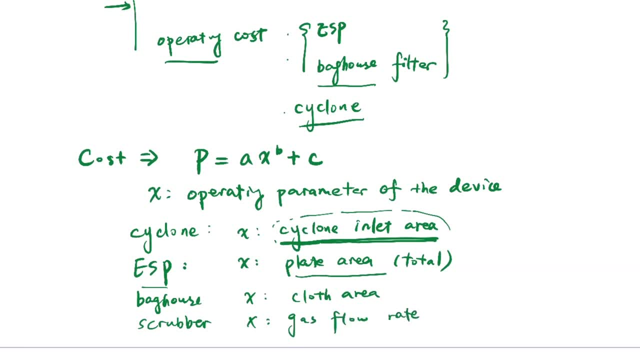 so, in general, we want to simplify this cost calculation so that we can- only we can- basically just refer to one type of the operating parameter and then to calculate this, this total price or total cost, here. okay, so i would say that maybe you guys can spend more time in your team project to. 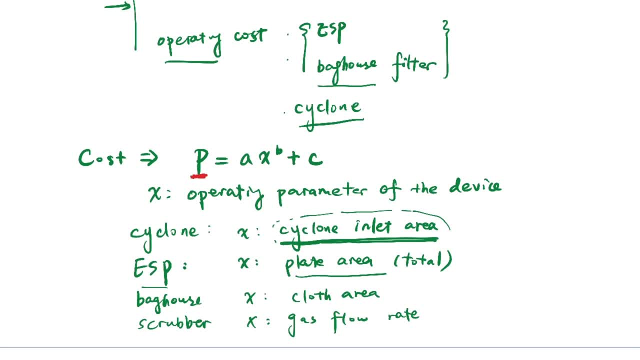 go through those final sections in each chapter about the cost so that you can get a more accurate estimation of the cost for each of these one or two week period. i think you know, let's say, for example, the total price of our cost of temperature then in pressurization. 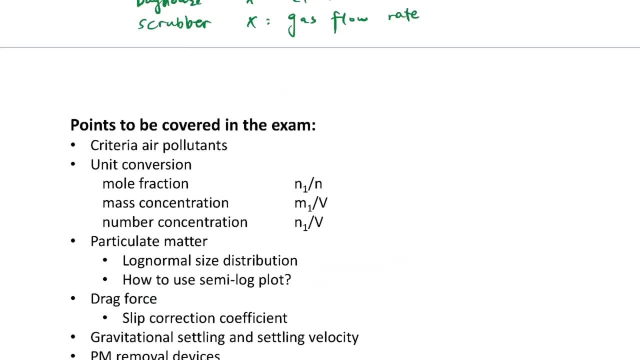 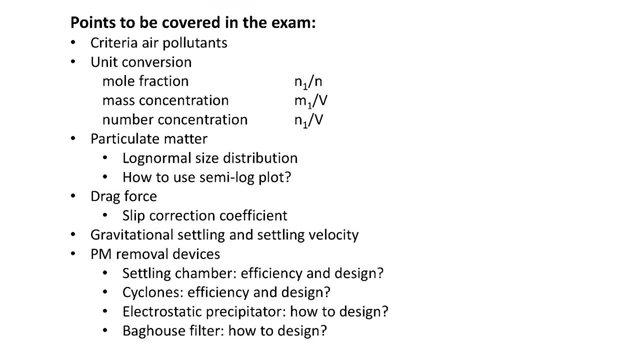 this is going to be based on the cost of the product, and so we can just see how it is going to be. so in general, you can see how the cost is going to be, and then the cost of the photo is going to be based on the cost of the product. 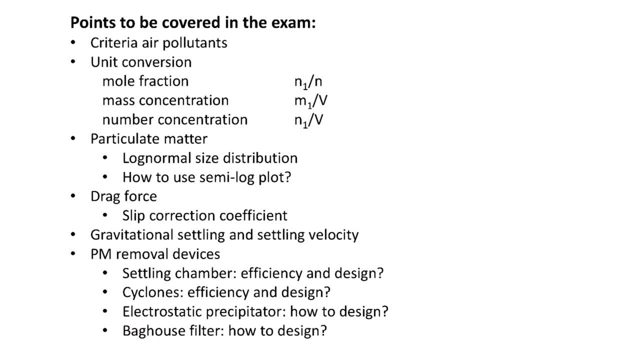 and then we will ask some questions about how is the cost of the product going to be? so this is the cost of the product, so you and your students are going to need to come to think about these for your devices covered in the exam, which are first, the criteria of air pollutants and also what are the first. 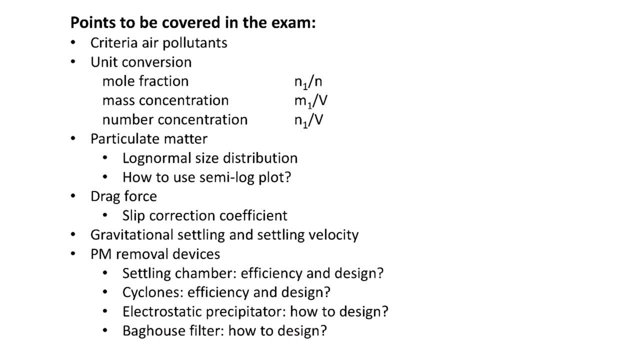 is the criteria: air pollutants, which are the most important types of air pollutants. So we have been mainly dealing with the PM. And then we know that there are sulfur dioxide, nitrogen dioxide, CO, lead and ozone. We further divide them into primary air pollutants. 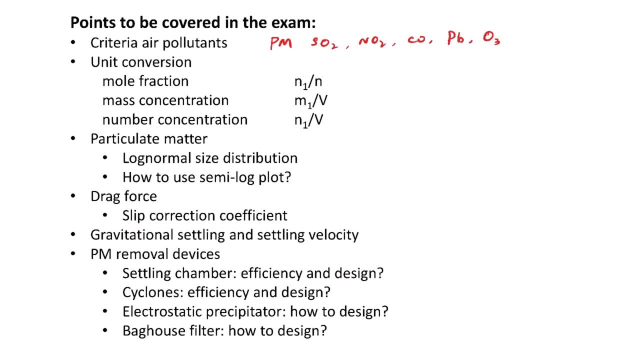 and secondary air pollutants based on how they're being formed. So we also introduced something on the air quality right, The air quality index. How do we calculate that, based on the concentrations of these air pollutants? And there was a quite important section on 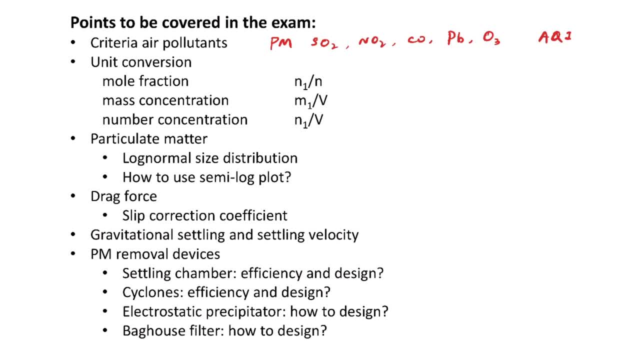 the in the introduction side. So until now we haven't talked about too much of it in the PM analysis, but later on, when we talk about the gaseous air pollutants, we're going to use this unit conversion quite often. Okay, So the unit conversion is basically using: 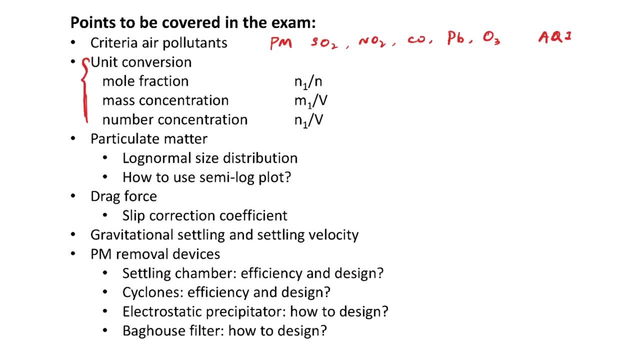 the ideal gas law to convert the quantities from all different types of units. Okay, For example, it can be mole fraction. You know that mole fraction can be having, can have the units of percent, right? PPP, PPM, PPM, so on, right. 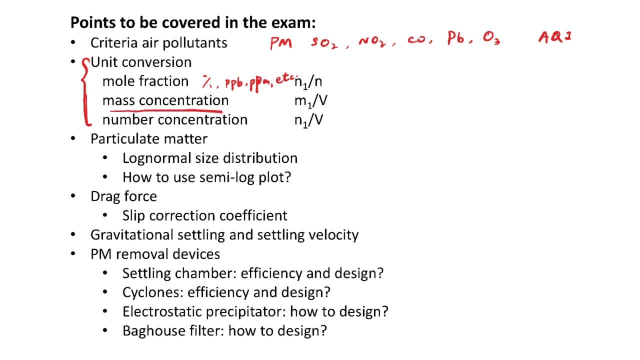 Mass concentration is going to be just be the mass of this, this single species, divided by the total volume. So those can carry the unit of, let's say, kilogram per meter cube or milligram per meter cube, so on right, And then we also have the number of concentration. 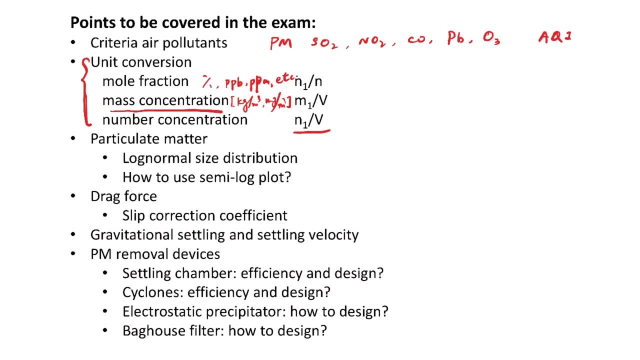 This is just the mole per meter cube, or number of molecules per meter cube. So what we're trying to achieve is basically converting from one another, right? I think in your homework, exam homework problems- you deal with quite many of these practice already, So here I just want to demonstrate this process. 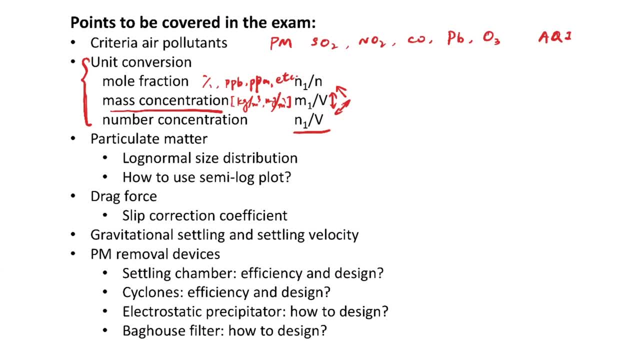 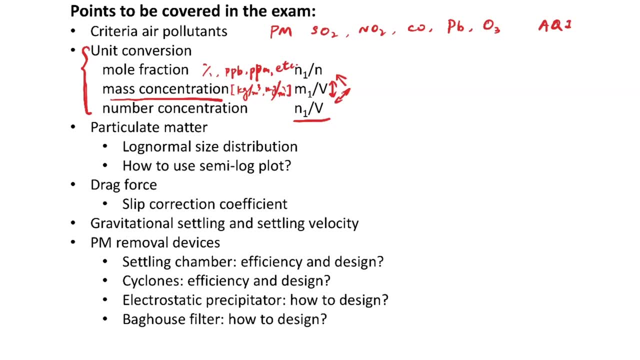 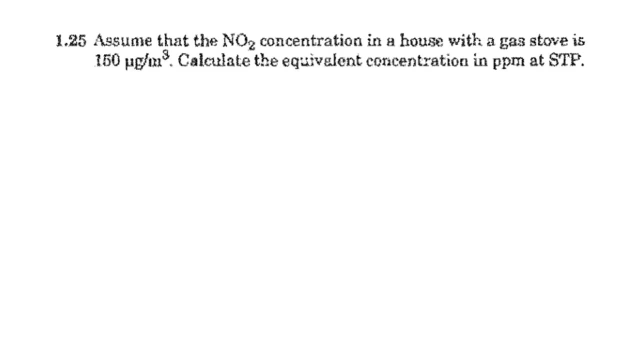 again, so that, so that is, if there's anything unclear for some of you, you can try to understand. how are we going to deal with this problem? Okay, So here I will show an example problem problem- And this is also one of your homework problem- This is 1.25.. And if you can find, 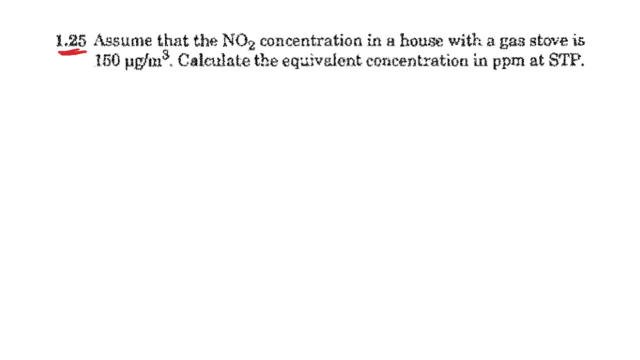 your previous homework, you can. I think now is also a good time to find it out, So let's just spend maybe one minute to read through this question and try to understand what it's asking us to do. Okay, So basically, it involves the nitrogen dioxide system and we want to. 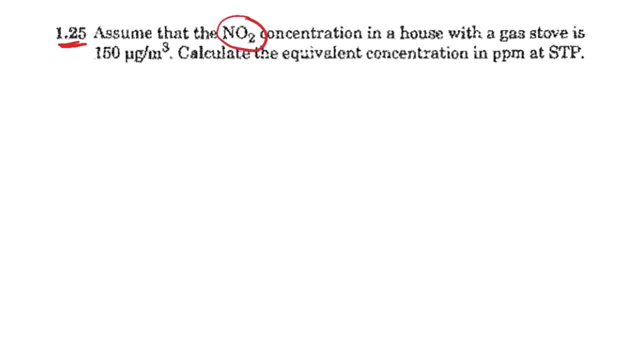 convert the unit from one to the other. So okay, I'll just read this problem now if you haven't gone through that. So assume that the nitrogen dioxide concentration in a house with a gas stove is 150 microgram per meter cube. It wants us to calculate what is the equivalent concentration in PPM. Okay, 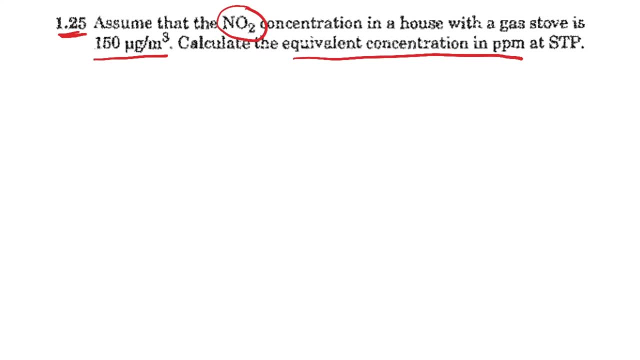 So just based on this problem problem, we know that it's actually trying to let us convert the mass concentration into mole fraction. This A here means this single species, and we're talking about nitrogen dioxide here. So we already have its mass concentration. we want to derive its mole fraction So as 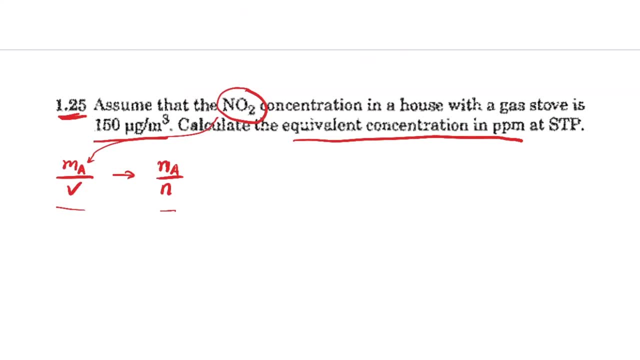 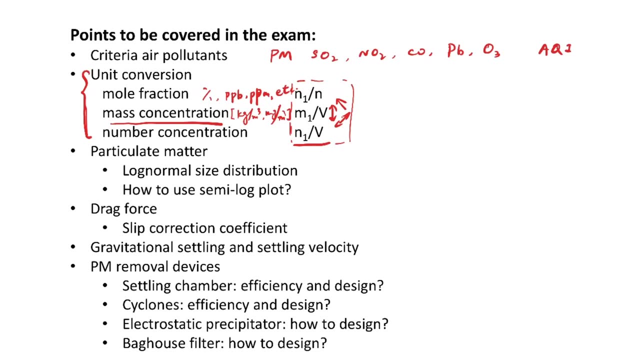 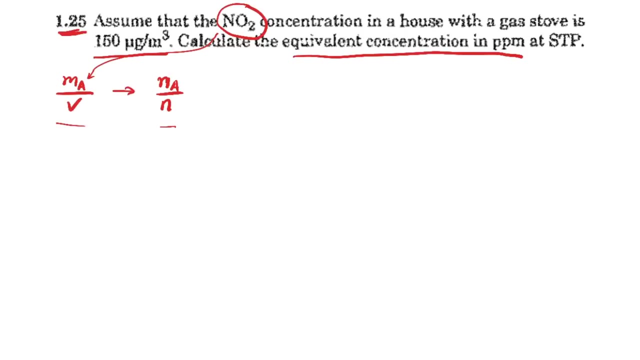 we have introduced here, we need to convert one from another in terms of the units. So how do we do that? I think during our classes I already gave those conversions from one to the other. I think if you have the class notes you can still find it. but here I'll. 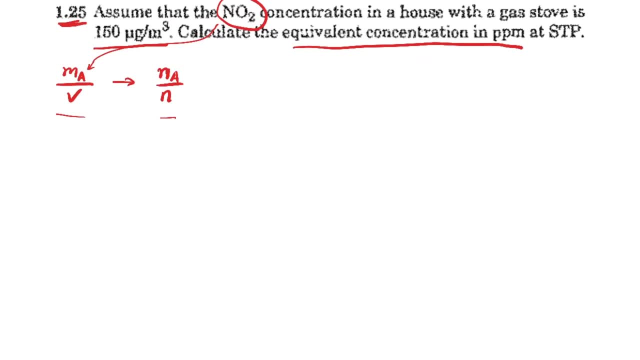 just try to redirect and derive it again. So we're trying to convert basically from an A to N, NA divided by N, NA divided by V and MA divided by V. So for these two it is quite straightforward, mainly because, let's say, if we build up an equation here, then we know that NA is equal. 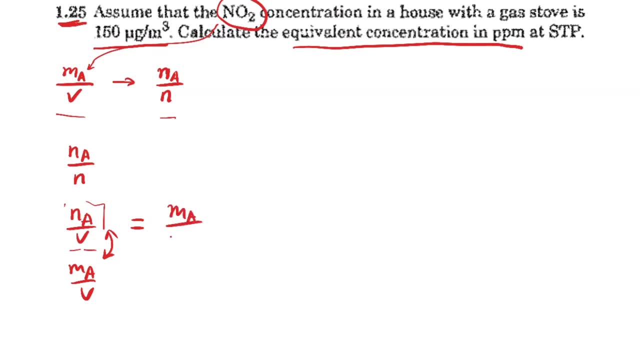 to MA divided by the molecular weight of A. So we can get MA divided by V multiplied by one over molecular weight of it. So in this way we can convert from the number concentration into the mass concentration. And then how do we convert from here to here? So we're 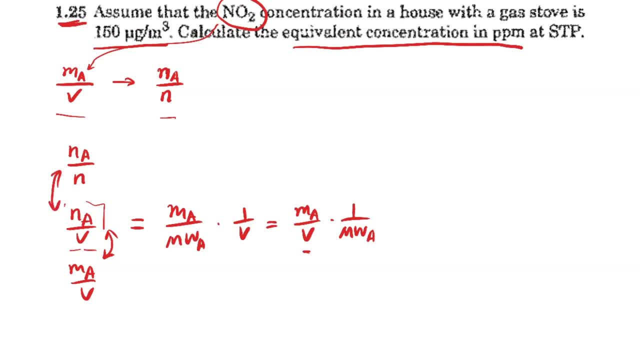 going to use the ideal gas law, which is PV equal to RT. We have N equal to, basically, PV divided by RT. So once we have this relationship, we can plug in this N here. So we have NA divided by PV multiplied by RT. So what we did is just plug in the N into this location. 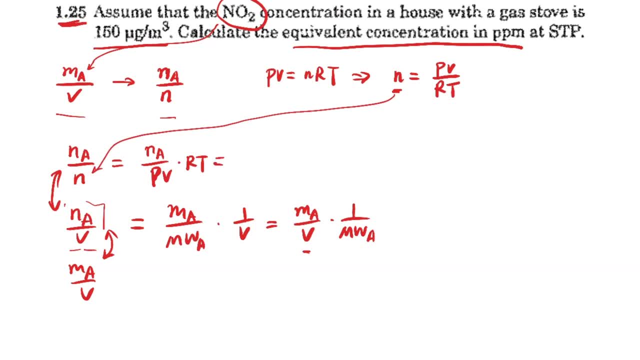 here. So we have NA divided by V, multiplied by RT, divided by P. So with this relationship, with this derivation, we can convert the mole fraction into number concentration And further we have number concentration into the mass concentration. We further plug that in MA, divided by V, multiplied by RT, divided by P, multiplied by the molecular. 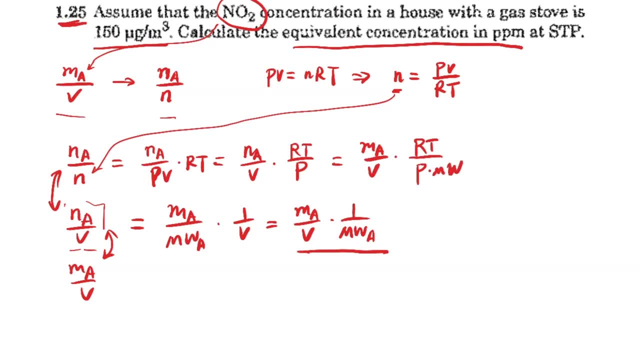 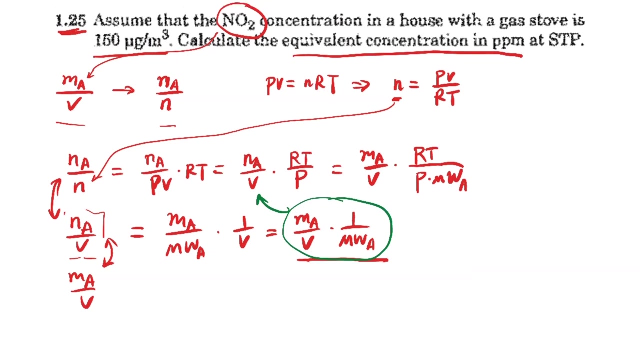 weight of it. So basically we're plugging in this term here into here. Any questions? Good, So basically now we have the equation which converts from the mole fraction into mass concentration, And then this problem wants us to calculate the mole fraction. 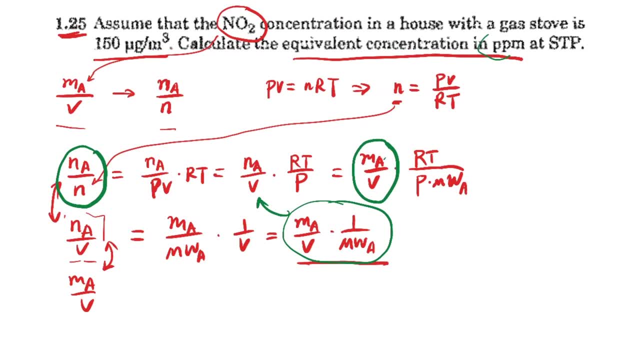 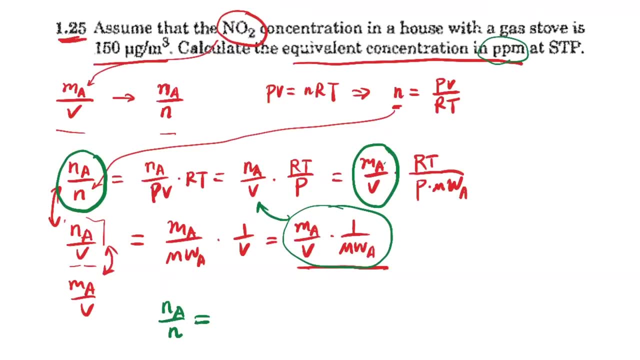 In PPM. So it is quite straightforward. We know that the NA divided by N is going to be equal to MA divided by V. We know that it's 150 microgram per meter cubed multiplied by RT. So RT is 8.314 joule per mole per k, And then, as standard, SDP means 273.14. 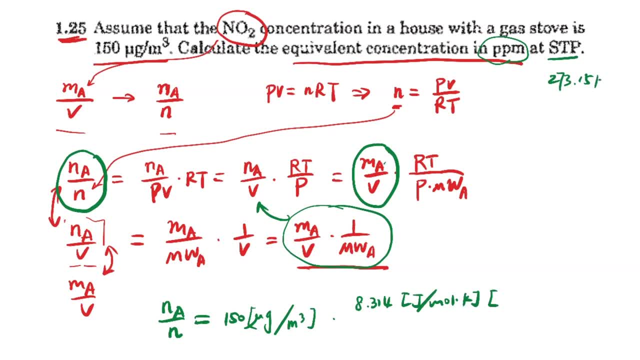 Okay, So we have 20.15 Kelvin and the pressure is 10 to the fifth pascal. Okay, So here we can just plug in this number of 273.15 k divided by 10 to the fifth pascal multiplied. 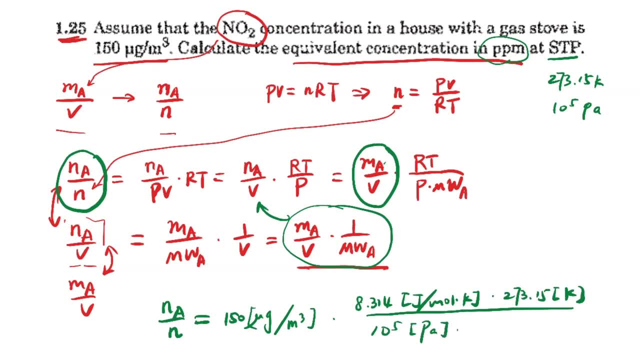 by the molecular weight. So for the nitrogen dioxide the molecular weight is basically 14 plus 2.5 Kelvin, 2 multiplied by 2, multiplied by 16, right, and that is 46 gram per mole. 46 gram per mole, and actually I think most of you have got to this step here. 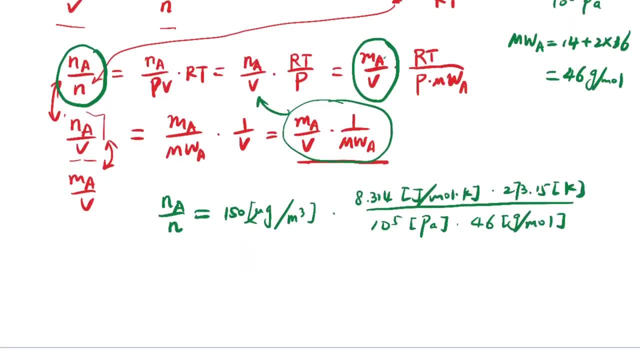 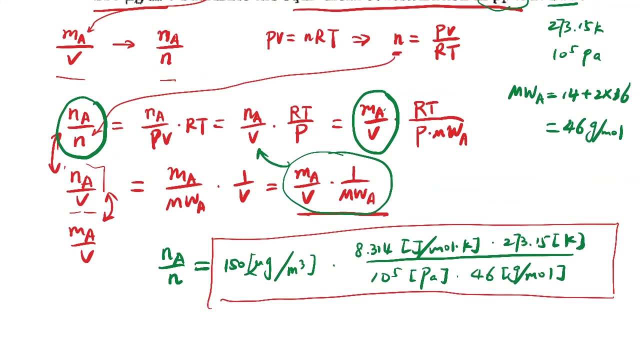 okay, so I know that there are very few of you who were using the equation in the textbook, so I would say that the equation- yes, excuse me, yes, you mentioned STP- that's mean the temperature- 25 Celsius and the pressure- 1 atom, right? so it really depends on which STP we're talking about, right? I saw that there are. 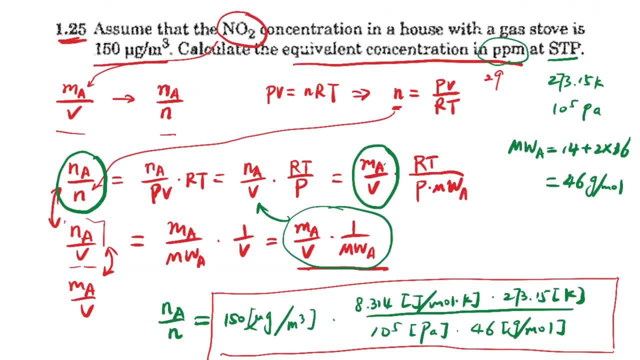 two types of STP. if I use this, it's correct: 25 Celsius the temperature and the pressure, 1 atom. it's okay, that's what. that's also fine. I would say that this problem is not probably not stated. well, yes, this is I mean also at this temperature and pressure. you'll 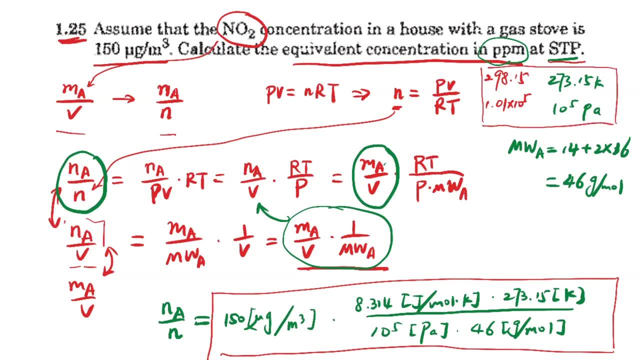 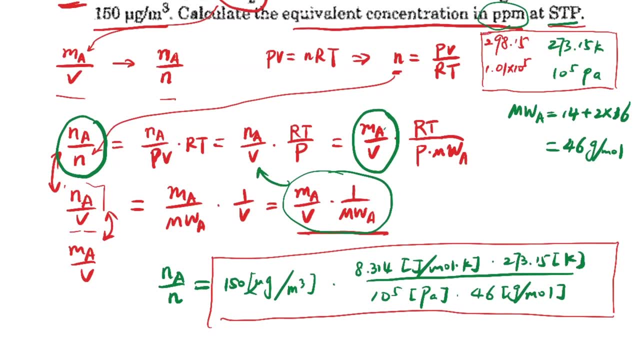 find out that it's not going to affect the final answer by a lot. okay, thank you. yeah, so in the future for these problems we'll just state clearly: what is the temperature, what is the pressure, right, any other questions? good, okay, so we're mentioning that there are maybe one or two of you who are using 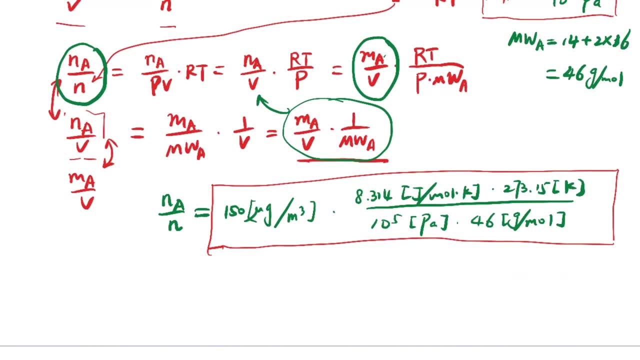 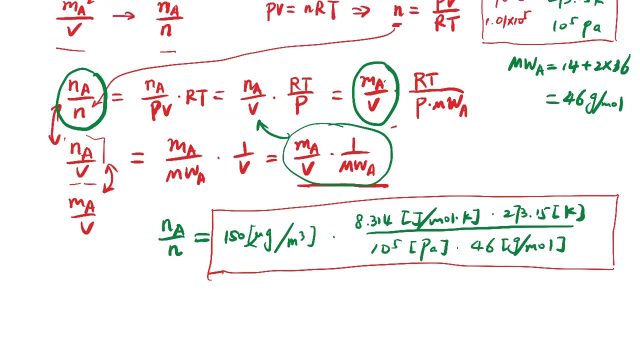 the equation in the textbook. so, the equation in the textbook, I would say some, it's a simplified version, but it's also having a lot of assumptions regarding temperature and pressure. I would say I would urge you to use this equation, okay, to use this type of relationship so that you can plug in the values more clearly. 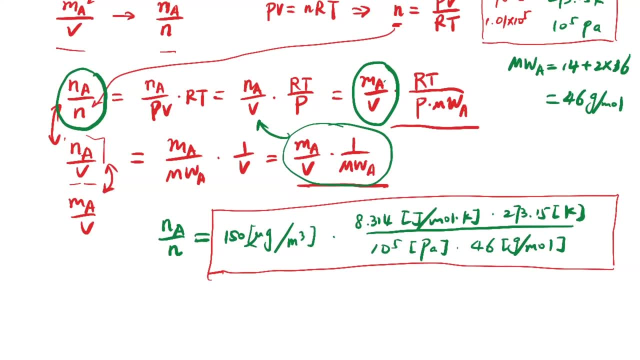 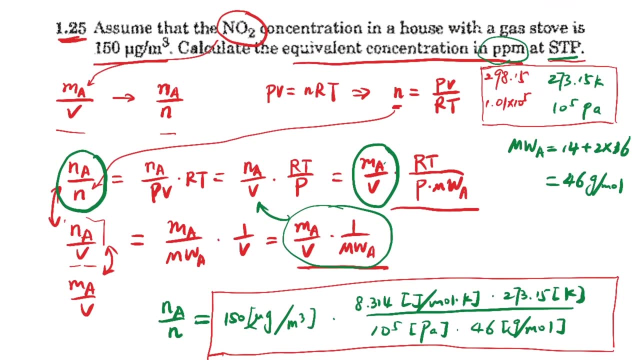 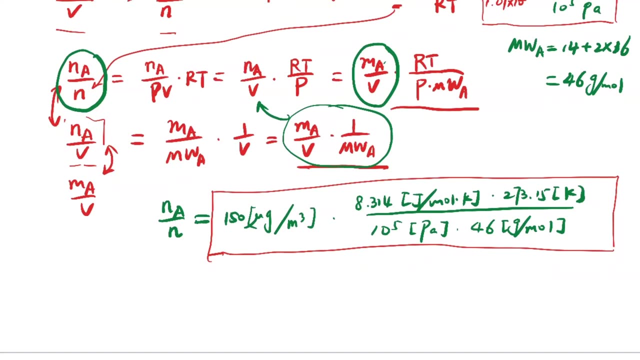 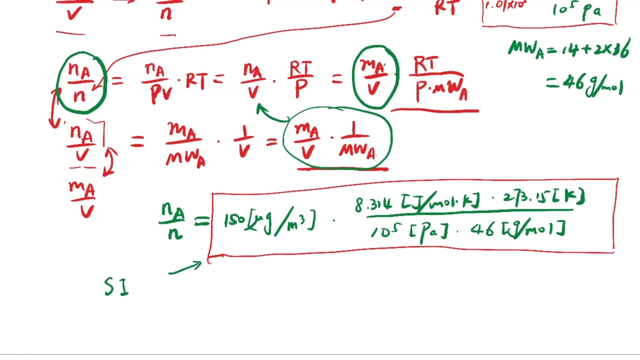 in there because there are. there's no assumption here except that we assume the gas will follow the ideal gas law, right? so basically, if you get to this step, the one important thing that you need to bear in mind is we need to use a standard unit. okay, so you need to unify all the units into the same setting for. 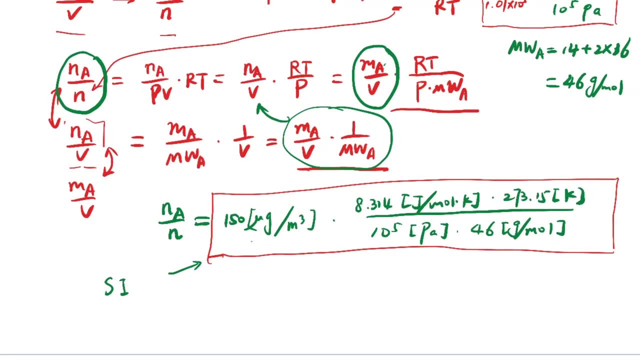 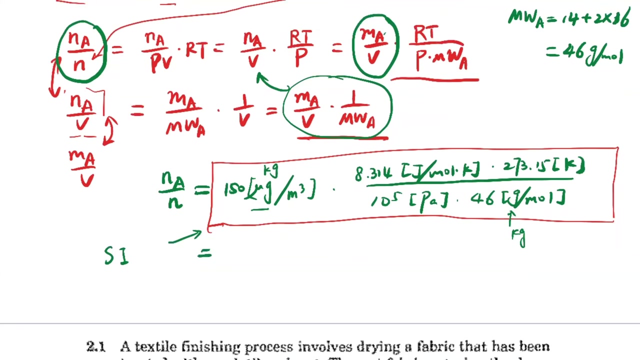 example the microgram per meter cube. this is not standard units. we know that for the mass the unit should be kilogram right. similarly, in here we shouldn't use gram, we should use kilogram right. so because of that we need to further do some unit conversion in terms of the detailed mass values. so this will be 150. 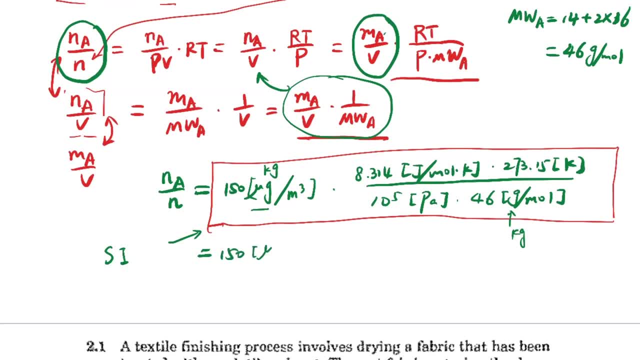 microgram per meter cube. so I saw that some of you prefer to use the method of just stating what is the relationship between different mass units. for example, we know that one kilogram is 10 to the ninth of the microgram right, so in this way you can cancel the microgram here. 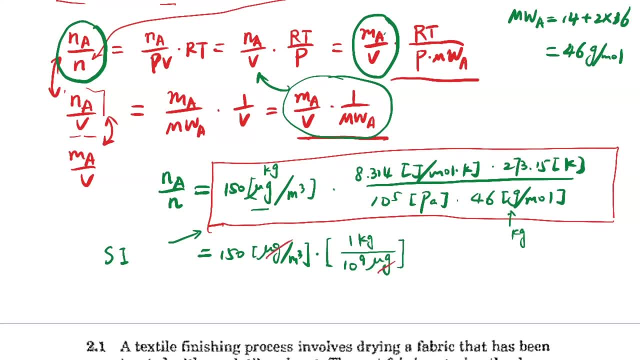 right. and then in this fraction here you have 8.314, still joule per mole, okay, and then 273, right, and then 273.15, 10 to the fifth passcode, and then for the molecule weight, that's going to be 46 multiplicity, 10 to the negative 3 kilogram per mole, okay, so now everything. 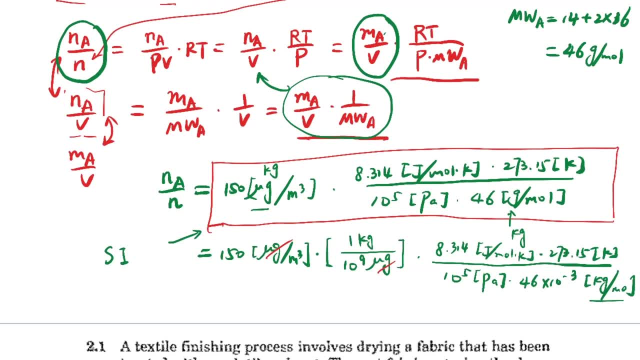 is in the standard units. we just need to use a calculator to happy in the values to find out. So the answer for this equation here is 7.4 multiplied by 10 to the negative 8,. okay, And we want to convert it into ppm. right, You know that ppm, we need to multiply that by 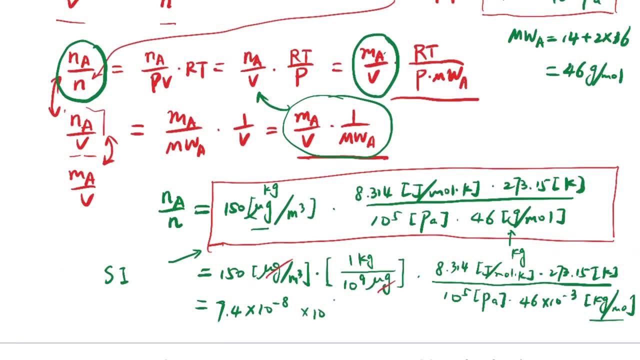 10 to the sixth. okay, Because it's parts per million. one million is 10 to the sixth, So that's going to be 0.074 ppm okay. So I would say there are two things that we need to pay attention here. So the first thing is to use this. 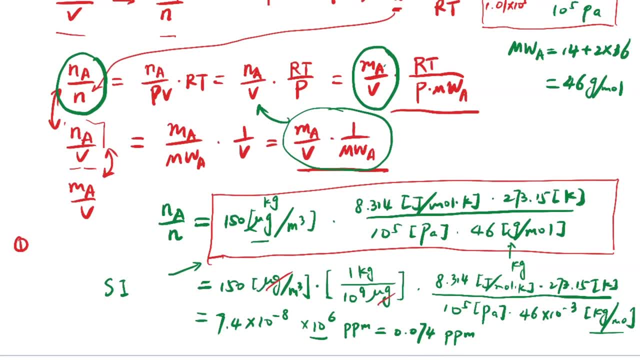 standard conversion equation here: okay, Use the correct equation, okay. And second thing is to use the standard units. So, if you can make sure that you're using the correct equation and also standard units, I would say that you should be able to get the 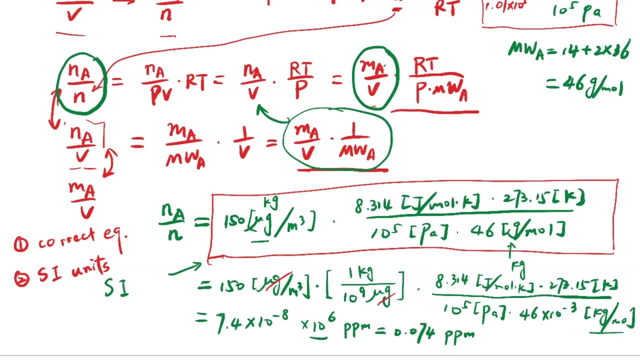 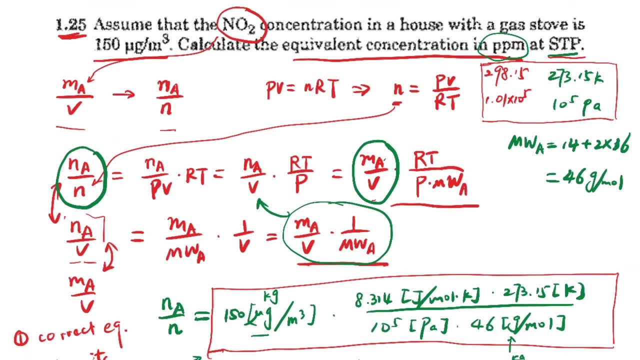 correct answer. okay, Try to practice more with this problem, because I often see that in the exam there are some, maybe quite a few of you that don't have any clue regarding the standard units. So I would say that you should be able to get the correct answer okay. 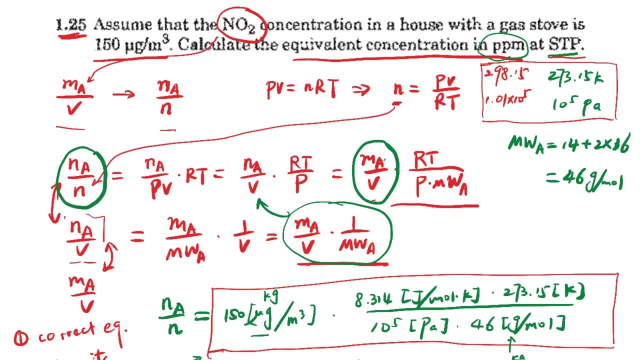 Try to practice more with this problem, because I often see that in the exam there are some of you that don't have any clue regarding this unit conversion problem, because this is quite an important topic, especially for the second half of the semester, right? So we want to make sure that you can understand. 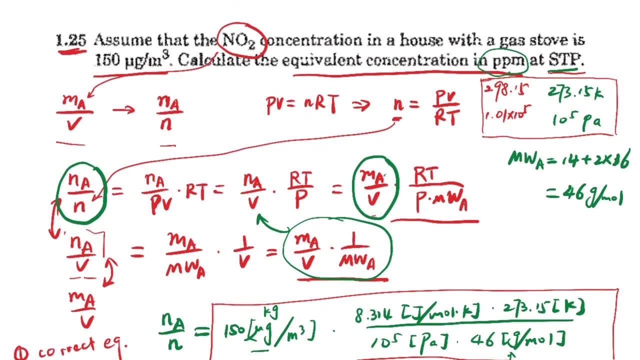 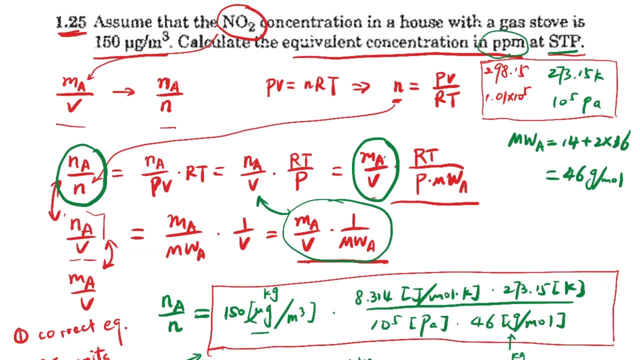 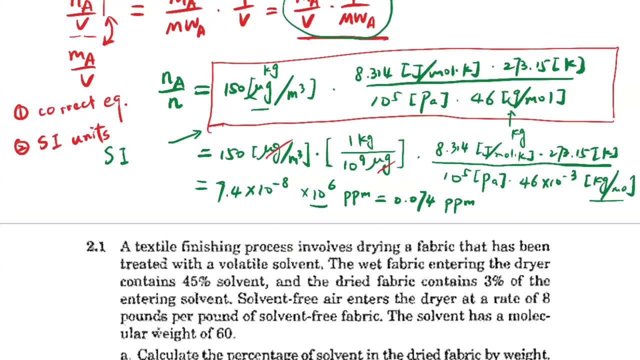 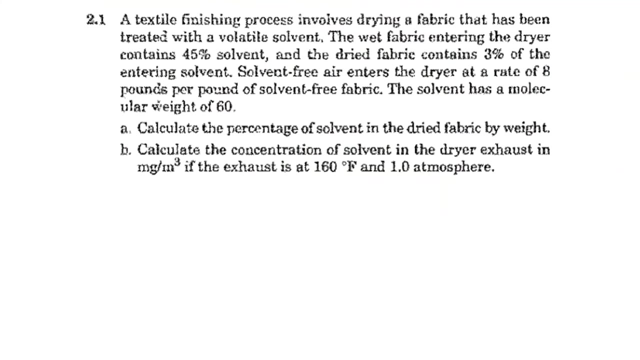 why are we going through certain equations to calculate this unit conversion problem right? So this is, I would say, a straightforward unit conversion, and there's also a problem that is not that straightforward, which is this problem here. It is quite, I'm quite happy to see that for this problem, quite many of you get the correct. 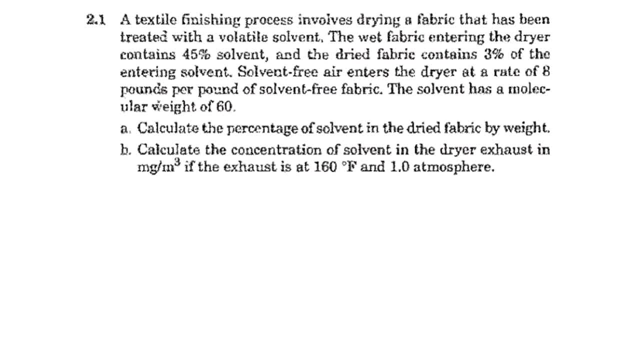 answer, I have to say that this problem is not stated very well. have to basically use your imagination to think about what is the drying process. So let's again spend maybe one or two minutes to read through this problem. All right, let's go ahead and read through this problem and see if there are any questions. 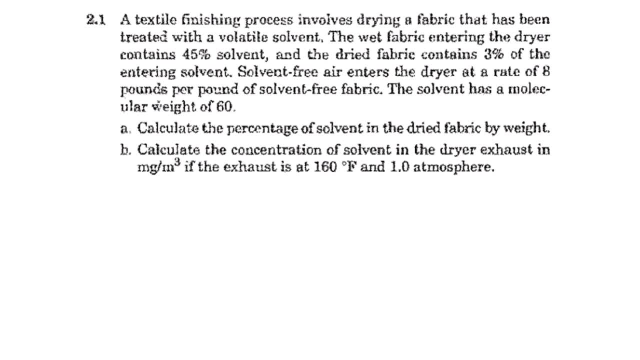 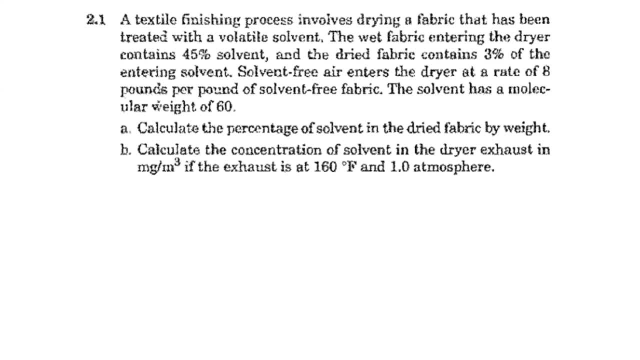 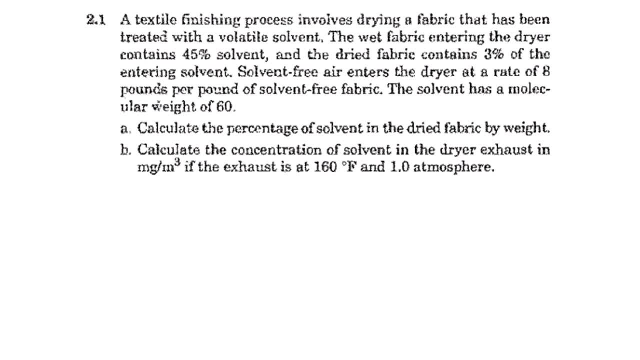 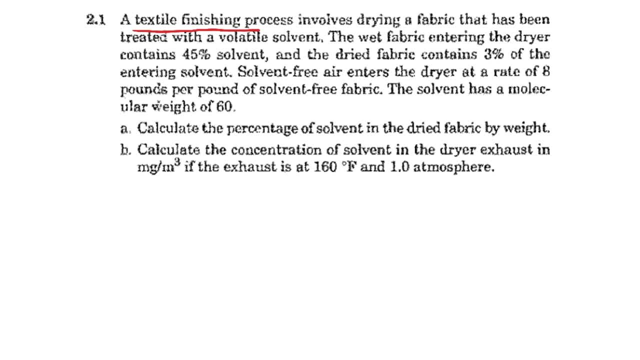 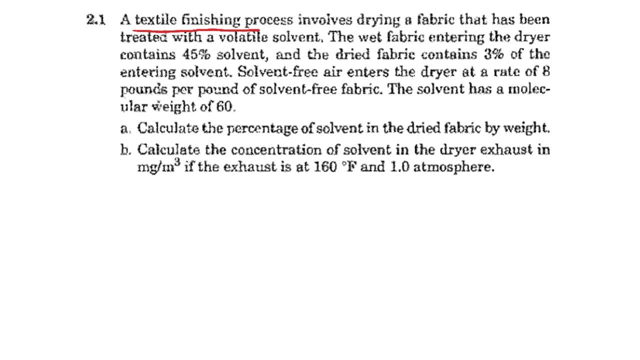 All right, All right, All right. a textile finishing process involves the drying of a fabric that has been treated with a volatile solvent. So this volatile solvent can be some, can be- some organics, right, because during the finishing of this textile we want to coat- maybe coat this cloth with some organics, right, so it? 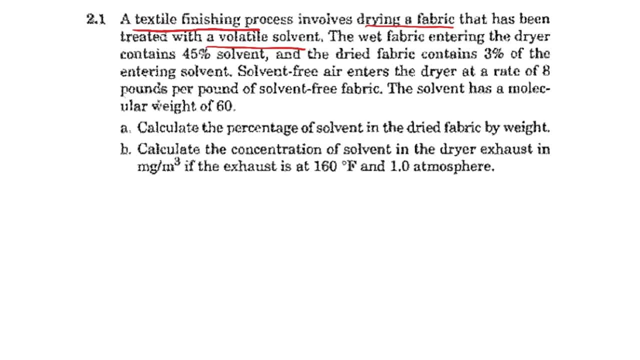 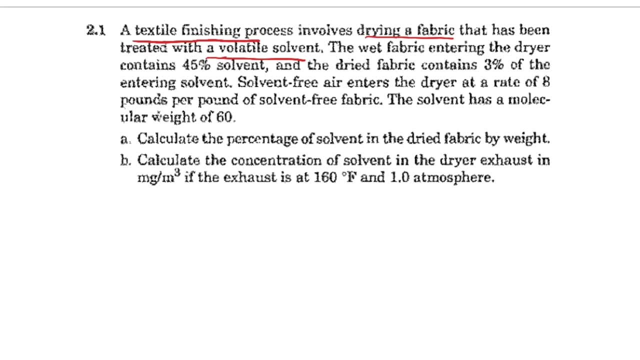 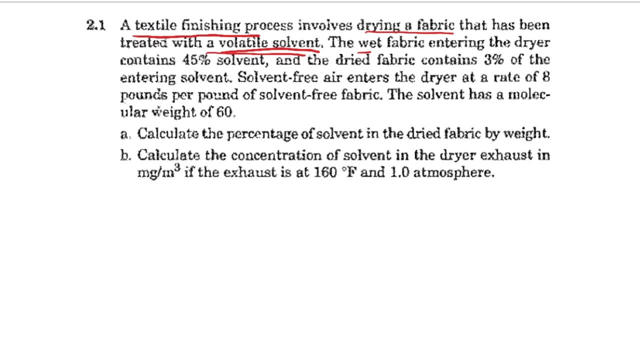 has a property that degrades less frequently, right, so it can last for a longer time. So this drying process tries to remove this extra volatile content. okay, so originally when we put them in there will be wet fabric. The wet fabric enters the dryer, but the wet 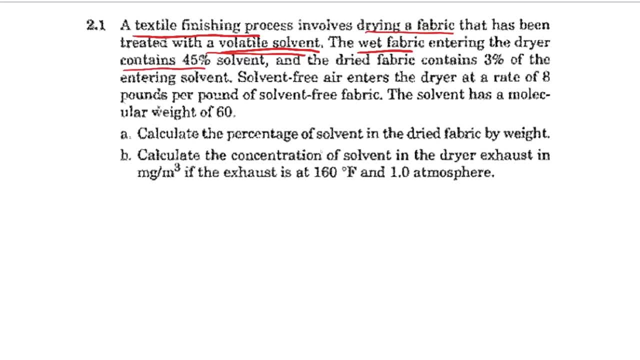 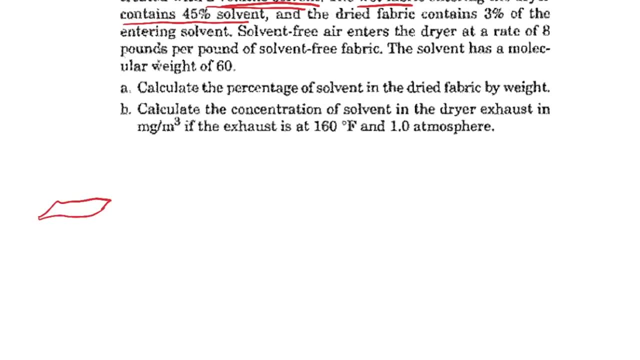 fabric also contains 45 percent of the solvent. So if we think about, let's say this is our fabric, okay, then we know that 45 percent of the mass are actually the solvent. So if we think about, let's say this is our fabric, okay, then we know that 45 percent of the mass are actually the solvent. 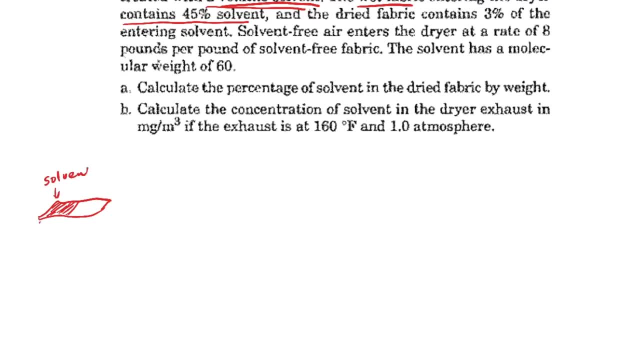 So if we think about- let's say, this is our fabric, okay, then we know that 45 percent of the mass are actually the solvent, Right? and then we're throwing that in to a dryer. Okay, so the wet fabric entering the dryer contains 45 percent of the solvent, and the dried fabric 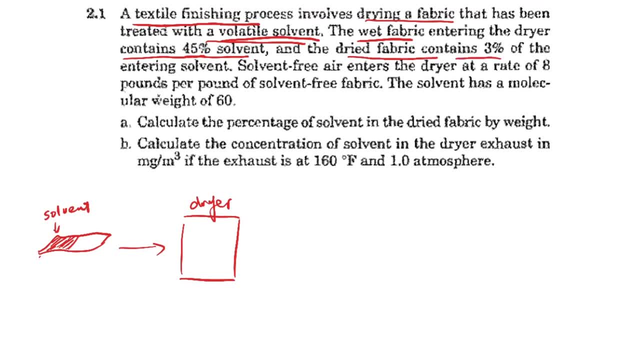 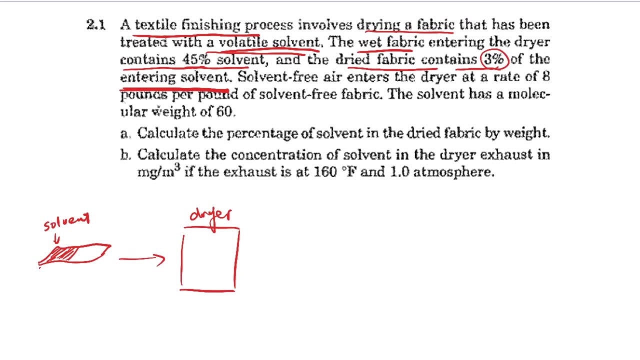 contains three percent of the entering solvent. Okay, so you can see that this three percent is not the final solvent concentration, but it's the three percent of the entering solvent. Okay, so if we set up a equation, set up a relationship regarding the properties of all the mass, let's assume that. 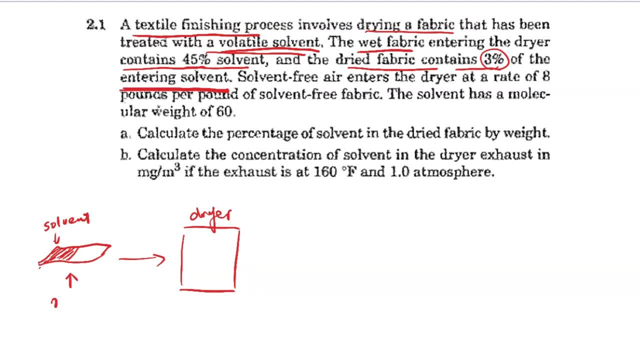 the original fabric mass is m. okay, I also saw some of you just use 100, let's say 100 kilogram or 100 grams. but that's, that is fine as well, because finally these numbers will cancel out. But right now, if we use a more general form, let's assume that the mass of the fabrics m, so we know that. 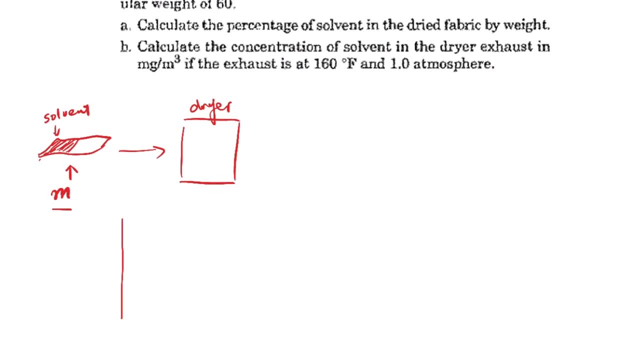 let's say this is wet, this is dry, right, if we put in the total mass, solvent mass and fabric mass, so the total mass- let's assume it's m- then for the wet fabric we know that the solvent mass will be 0.45 of m. 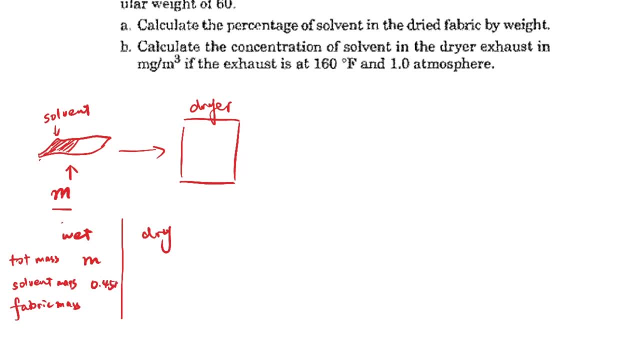 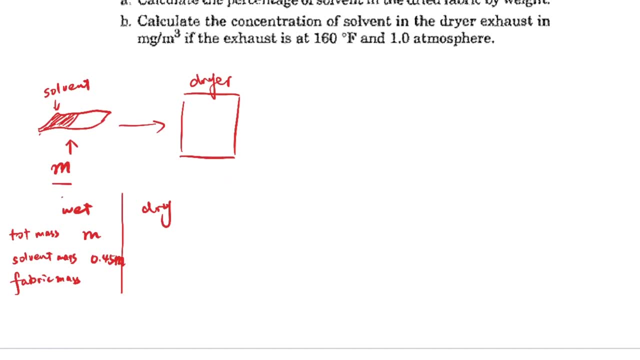 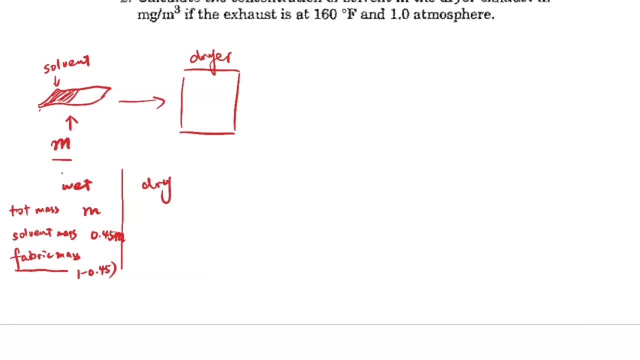 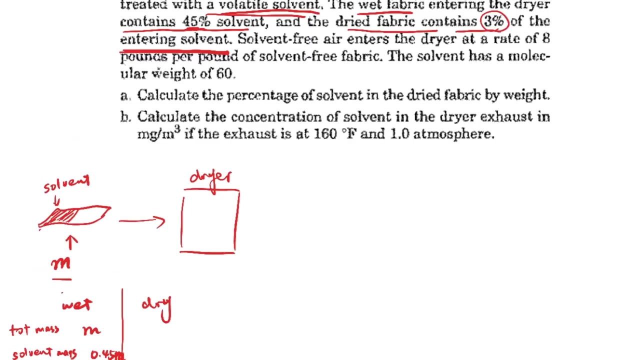 because it occupies 45 percent of the total mass. so, because of that, we know that the fabric mass will just be 1 minus .45 of m, right? because other than the solvent, it's just a dry fabric, right? so this is the fabric mass and we know that for the dried fabric, it contains three percent of the. 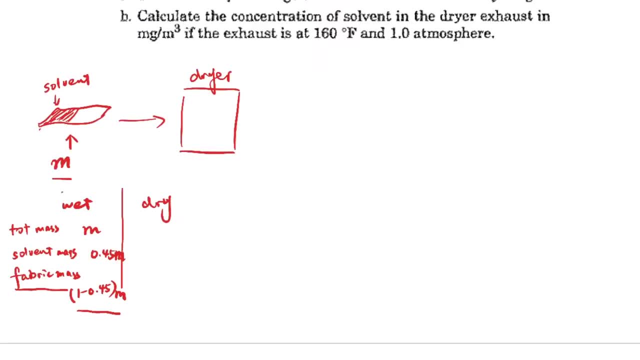 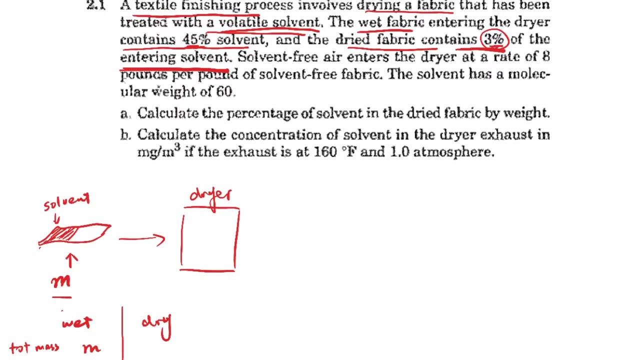 original entering solvent. So we know that for the dry fabric, the solvent mass will be 0.45 M multiplied by 0.03.. So this is what the problem stated: It contains 3% of the entering solvent And then the solvent-free air, which is the dry air going through this dryer. 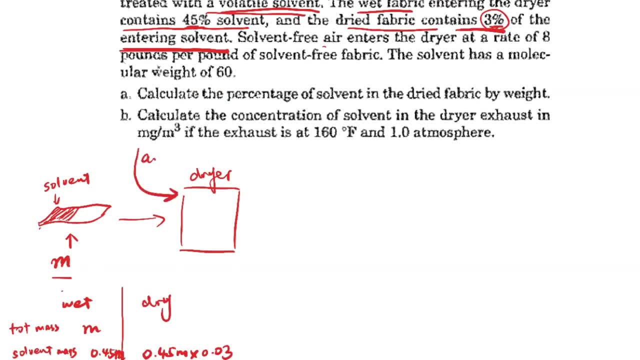 The air enters the dryer at a rate of 8 pounds per pound of solvent-free fabric. okay, So what that means is for every one kilogram, let's say every one pound of the dry fabric, of the dry fabric is referred to this area, So let's use another color here. 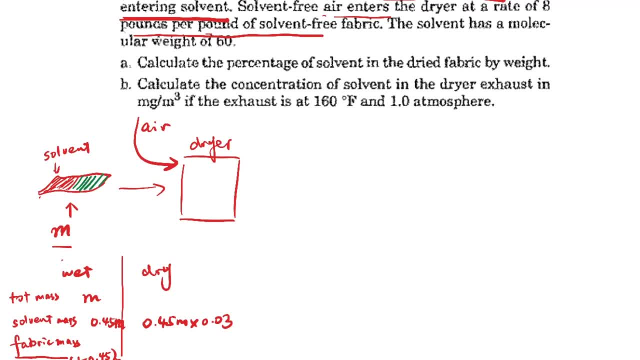 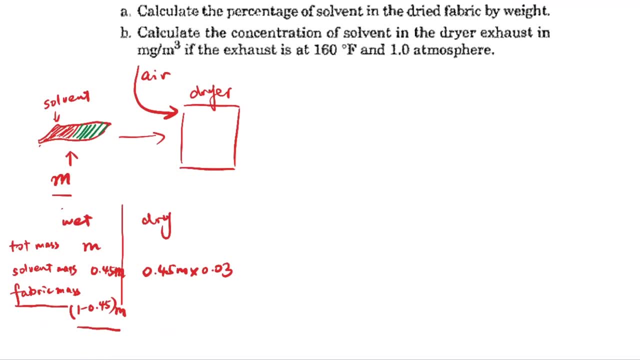 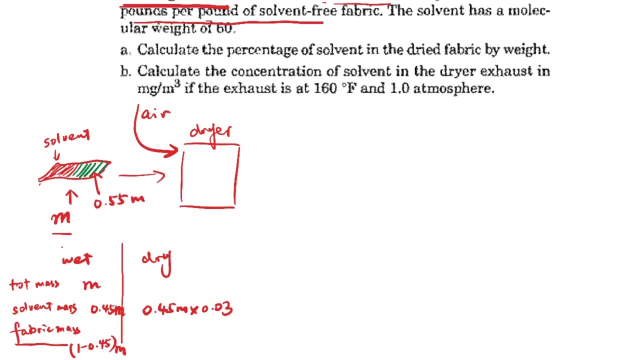 So for every one pound of this dried fabric, we have 8 pounds of the dry air, right? So what that means is we know already that this dry fabric is 0.55 M, So the amount of air that enters the dryer will be 0.55 multiplied by 8 of M. 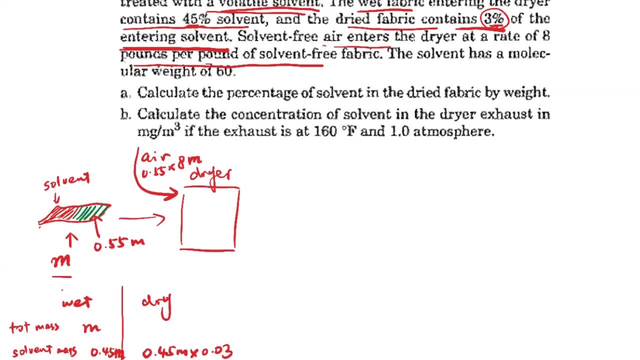 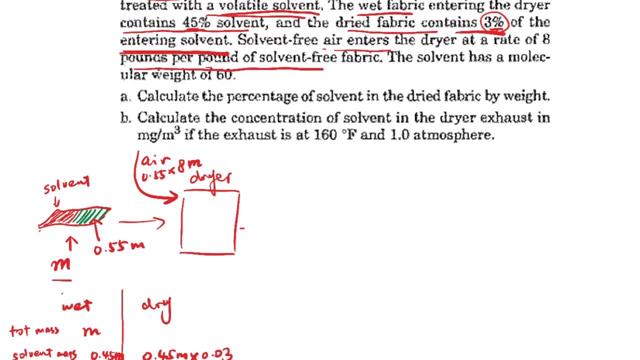 Right, So this is how we can calculate the mass of the air entering the system. Okay, so we know that. finally, when the fabric come out, this we call it dry fabric, but still it contains some quantity of the solvent, and then we have the wet air. 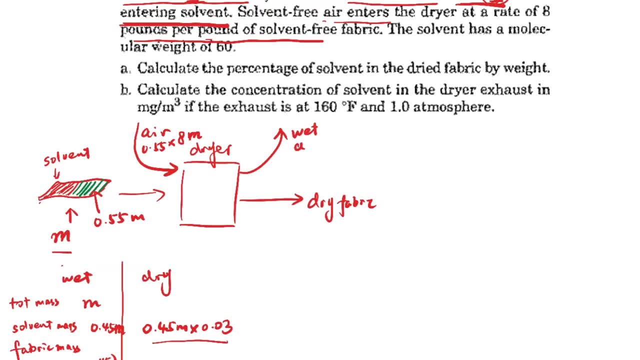 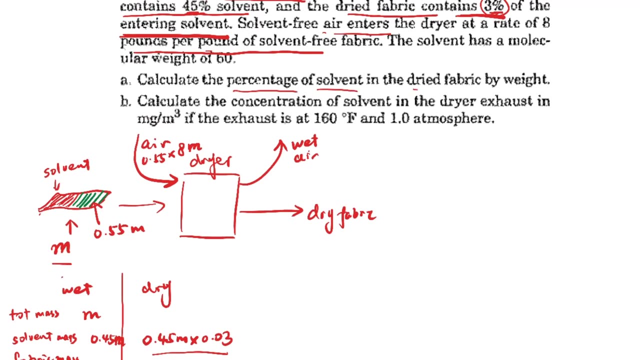 coming out, which is basically the solvent, are being picked up by the dry air from the system, right? So now let's see what this question asks us about. So it first wants us to calculate the percentage of the solvent in the dryer by the dry fabric, by weight. okay, 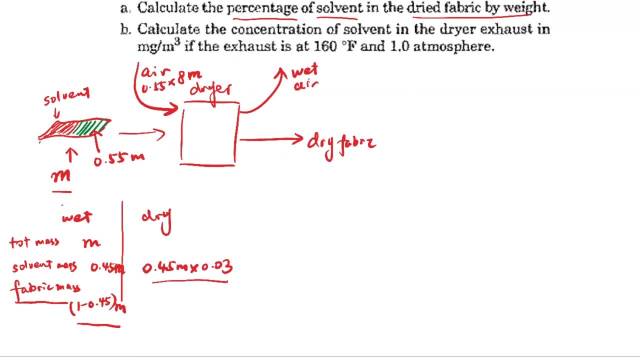 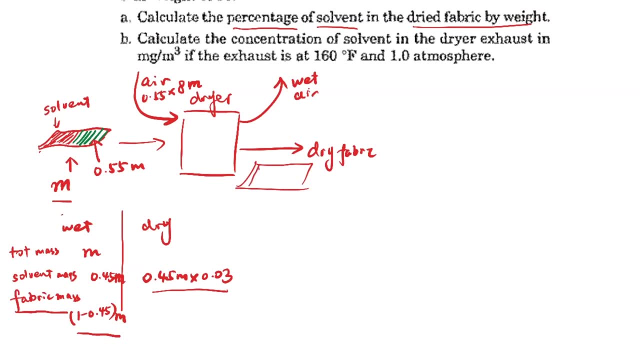 So basically it wants us to calculate. let's say, this is a dry fabric, still dry out. okay, So now we know that after drying, the fraction of the solvent will be very less and then most of it will just be the dry fabric, right? 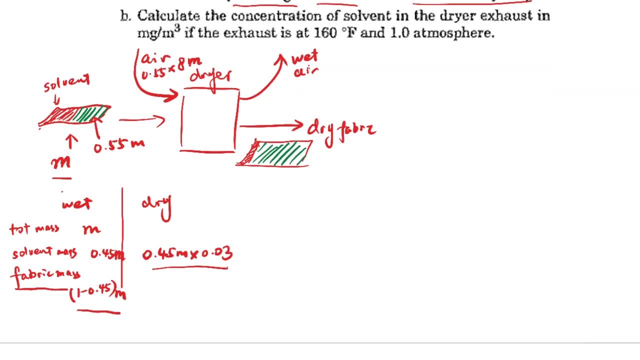 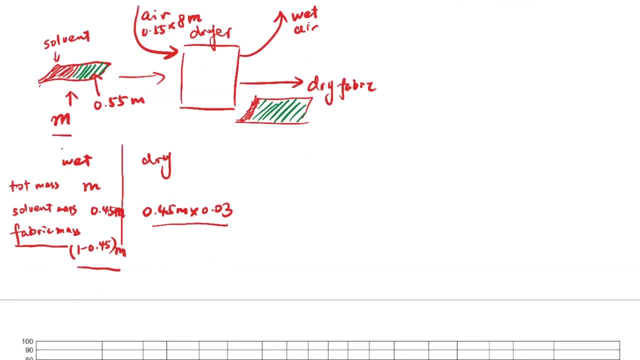 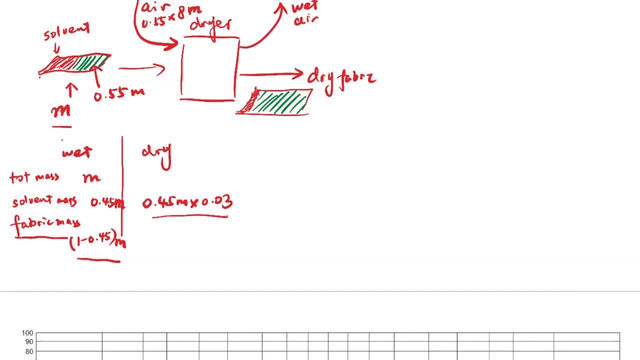 So we just need to know what is a fraction, the mass fraction of the solvent. So we have already shown here, this table here, that the solvent mass in the dry fabrics is three percent of the 0.5 m right, but at the same time the fabric mass will not change at all. it's not like dry after drying the fabric. 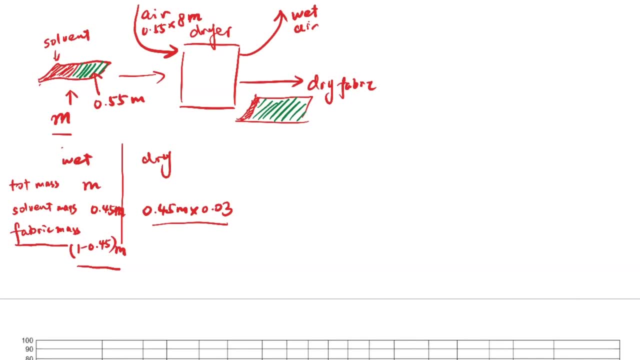 also lose some contents there. so the fabric is still in its original mass. we know that this is still going to be 0.55 of m. okay, so based on these two we can calculate what is total mass as 0.55 plus 0.45 multiplied by 0.03 of m. okay, so to calculate what is the percentage of the solvent. 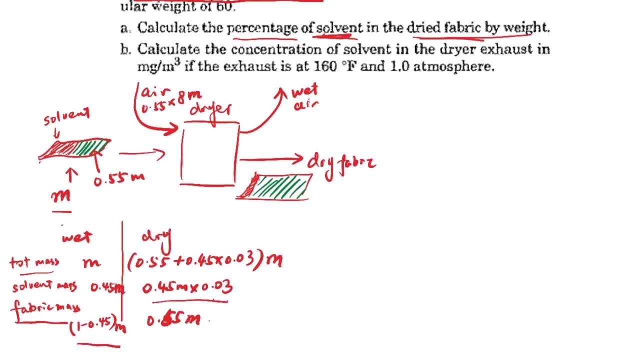 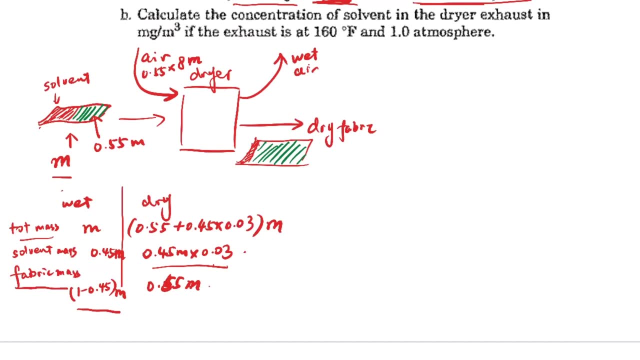 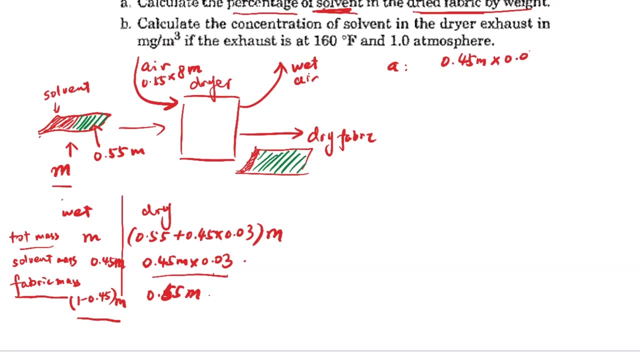 in the dried fabric, then we can just divide this solvent mass by the total mass, right? so for this a here we just need to plug in 0.45 m multiplied by 0.03, divided by 0.55 m, plus say, if we take the m outside, 0.55 plus 0.45 multiplied by 0.03. 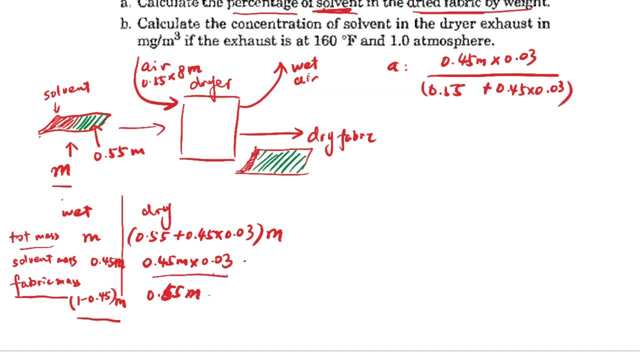 of m. okay, so we mentioned that you can either plug in 0.45 m multiplied by 0.03 of m. okay, so we mentioned that you can either use 100 as the mass, or you can use 1 as a mass, or you can use, let's say, you can. 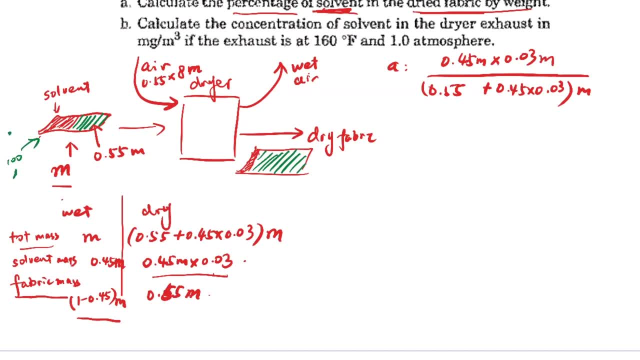 even use PI as the mass, right? so any mass, it doesn't matter, because finally they will cancel out here, right? so if you again use your calculator to check what the answer is, so the final answer is 0.0076, which is 0.76 percent. 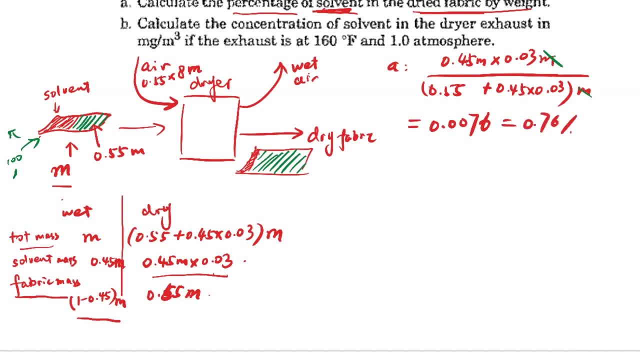 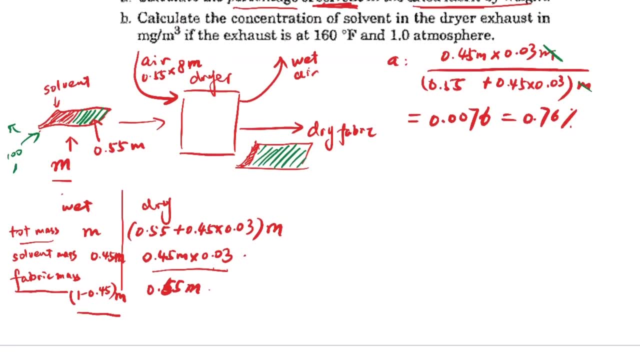 okay, so this is how we calculate the percentage of the solvent in the dried fabric right. so basically, it's using the mass conservation, that the fabric mass is not going to change right during this dry process, while the solvent mass reduced, mainly because we're drying the fabric right. and then, secondly, it wants: 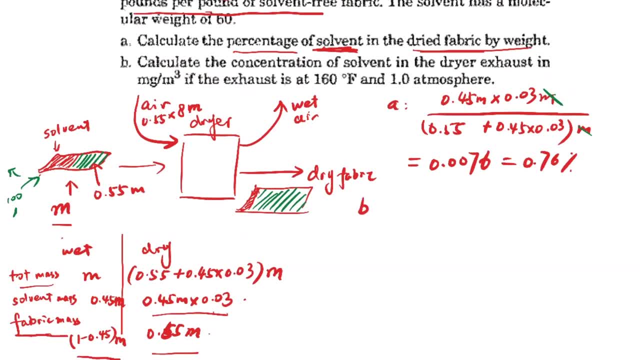 us to calculate the concentration of the solvent in the dryer exhaust in milligram per meter cube right and also give us the condition of the environment, which is at certain certain temperature and certain pressure. okay, so if you check what this problem asked us about, it asked about a mass. 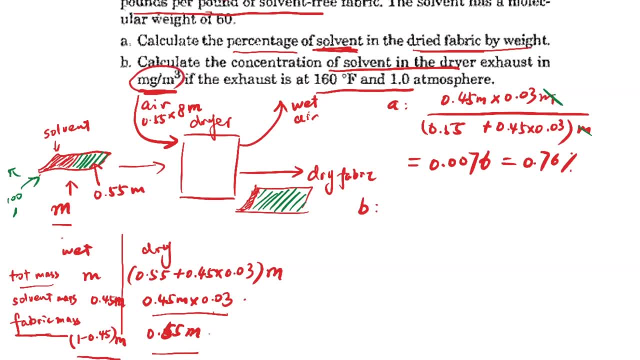 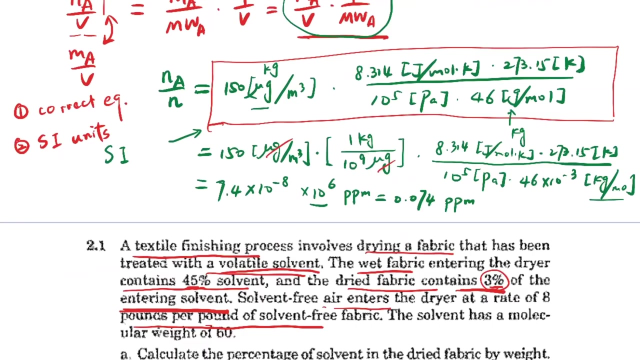 concentration of the solvent in the air, right? basically, it's asking us about the MA over V. that's why it's having the unit of milligram per meter cube. okay, so it may be quite difficult to directly get this quantity here, but we have introduced that these things can convert from one another, right? so what? 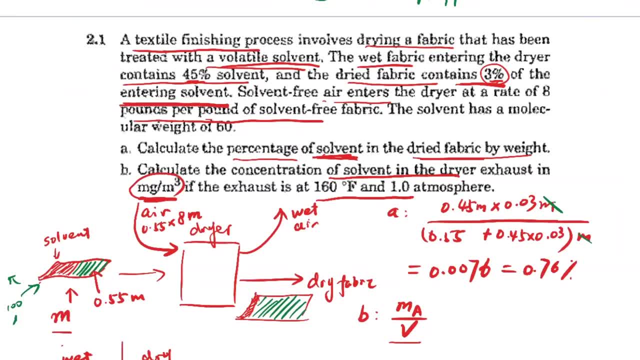 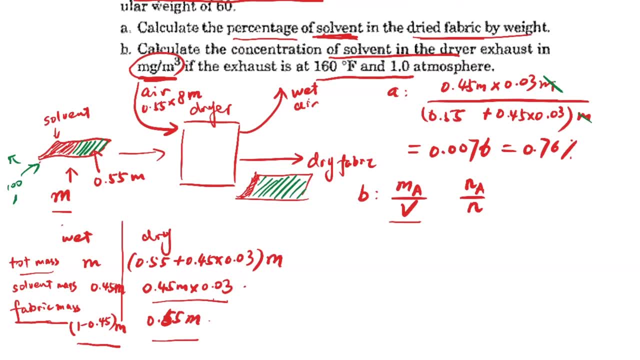 about NA divided by N. so NA here is the, basically the moles of the solvent in the air, and N here is the total number of moles of the air. so see what conditions we already have. so we have, basically we know what is the mass of the solvent in the dried. 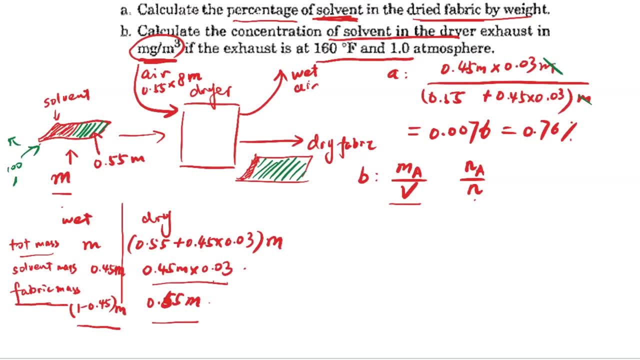 fabric. right, so we know that the solvent in the air will just be 97% of the original solvent amount. right, that will be 97% multiplied by 0.45 M, because we only have three percent of the original solvent mass in the fabric. so you will just entre gauge of the active solvent in the one edge of the 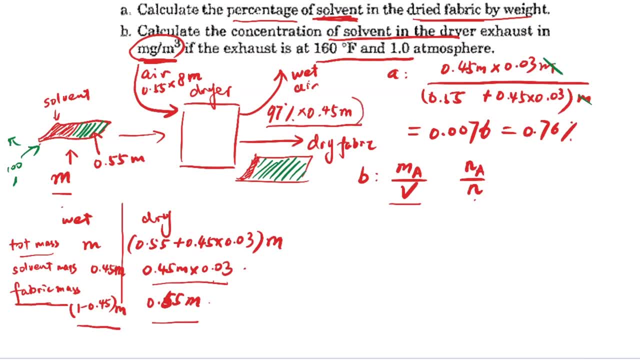 fabric, right? so 97 percent of the solvent will be in the wet air. right, so we know what is the mass of these solvent in the wet air. if we know the mass, we can just divided that by the molecular weight of a to calculate what is the number or what is the mose of a right. so what about the total number of? 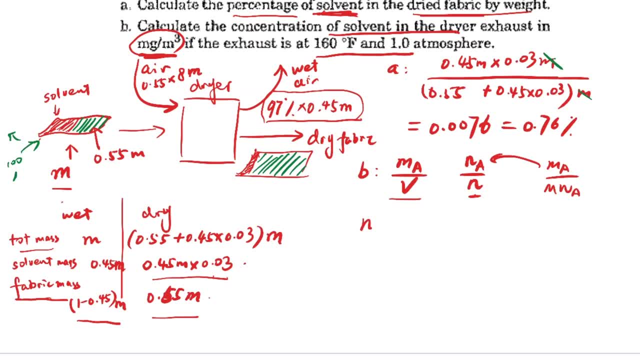 So we know that n the total number of moles will be equal to nA plus n of the air. right, So nA. we can already solve that because we know the mass of the solvent. we can divide that by the molecular weight to get nA. 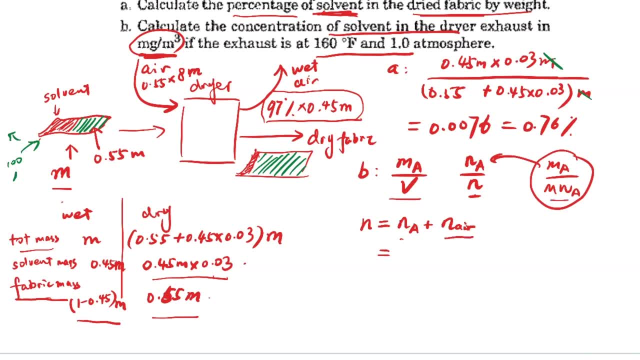 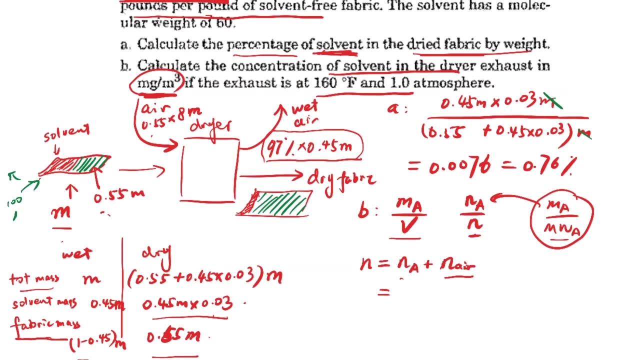 And for the n air, we also know the air, we also know the mass of air that's entering the system. right, We already know that for each pound of the solvent, so for each pound of the dried fabric, we have eight pounds of the air right. 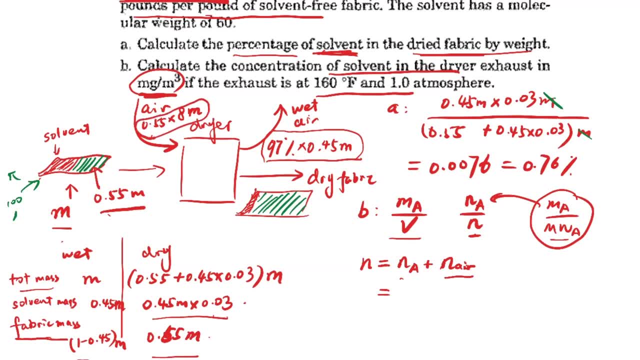 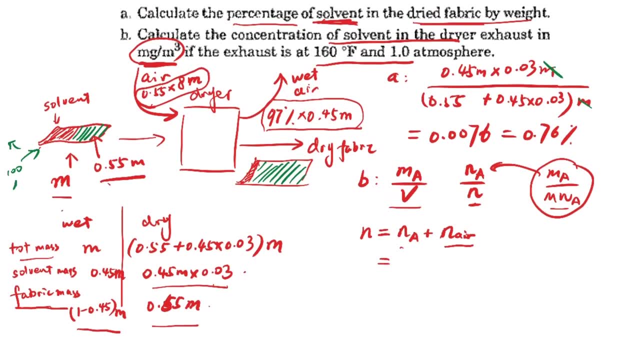 So, based on the mass of the air, we can calculate how many moles of the air molecules are there. right So this? because of that, we can solve for this problem. right So, mA? we already know that it's 0.97 multiplied by 0.45.. 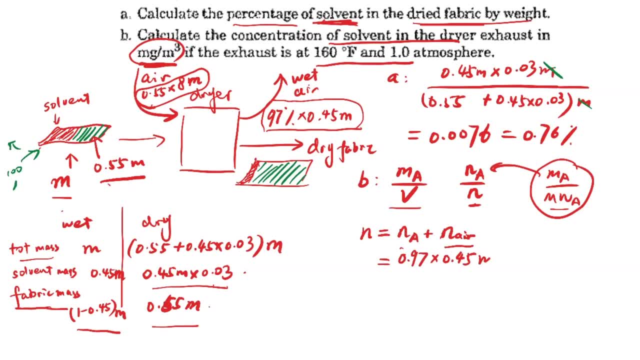 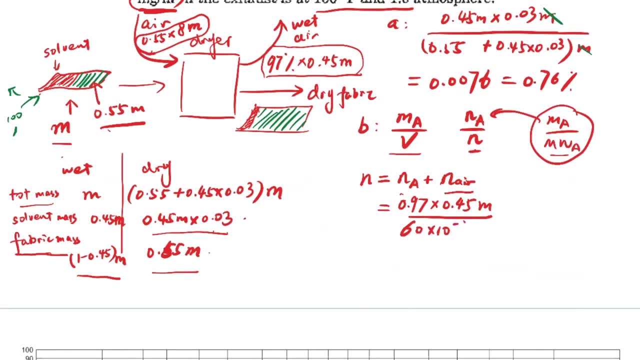 mA divided by the molecular weight. the molecular weight it already gave us is 60, right, So 60 multiplied by 10 to the negative 3, right Because we still need to use the standard unit, which is kilogram per meter cube. 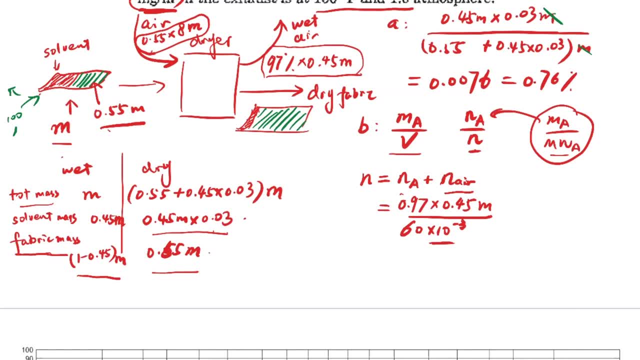 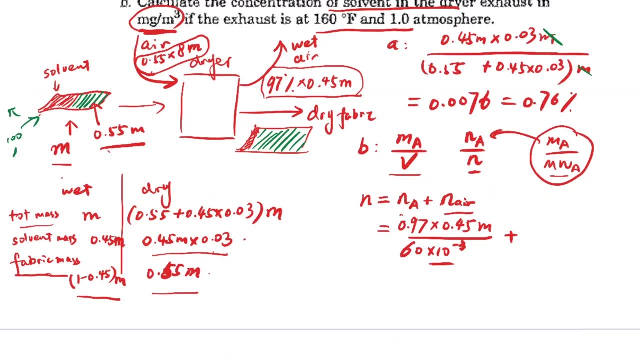 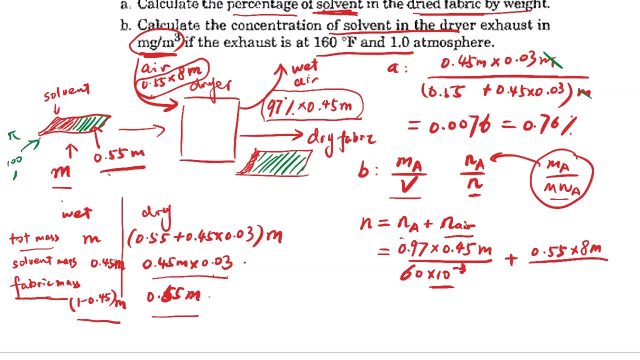 So this is the number, this is the moles of the solvent. In terms of the moles of the air, we have 0.55 multiplied by 8 of the air, And then we'll divide that by the molecular weight of the air, which is 29 multiplied. 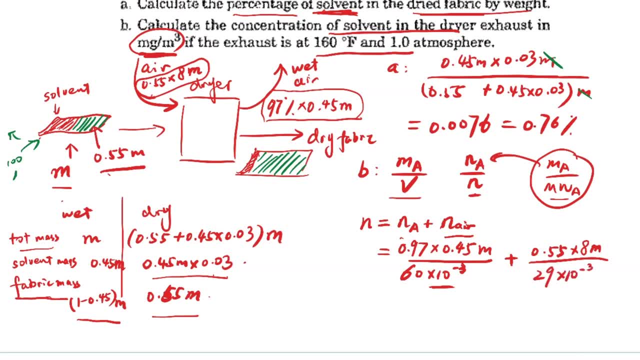 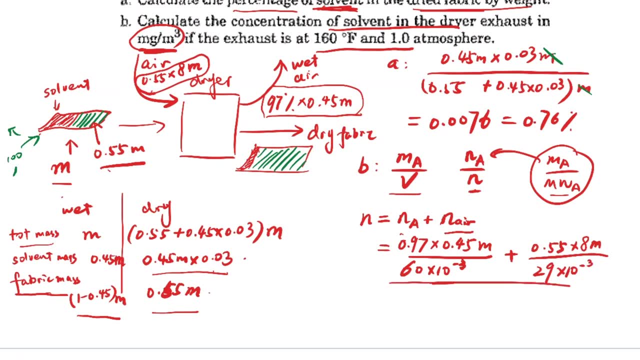 by negative 3, also kilogram per mole, right? So with this quantity here we should be able to calculate what is the total moles of the species in this wet air here, right? And we already know what is the mA. 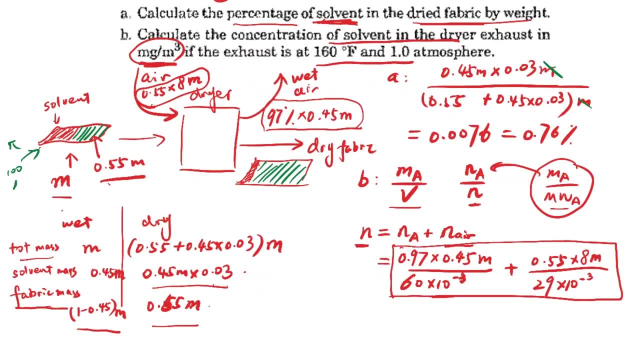 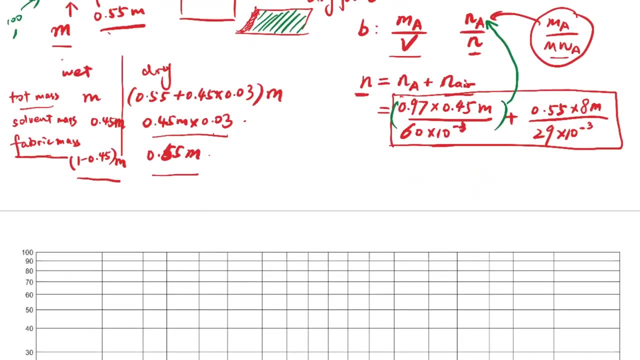 Right, mA is just this. it's just this first term here, right? So basically we can plug in these values And again these m will get canceled out. We can find out that mA divided by n is actually 0.0458, okay. 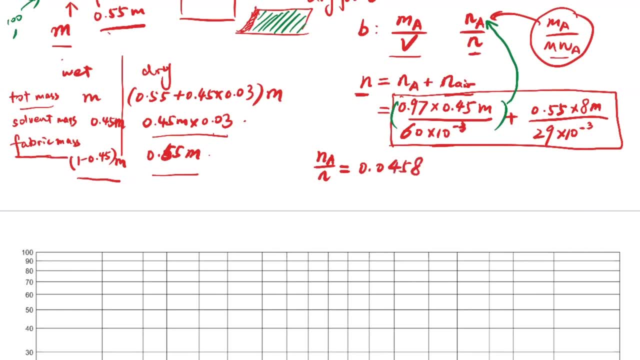 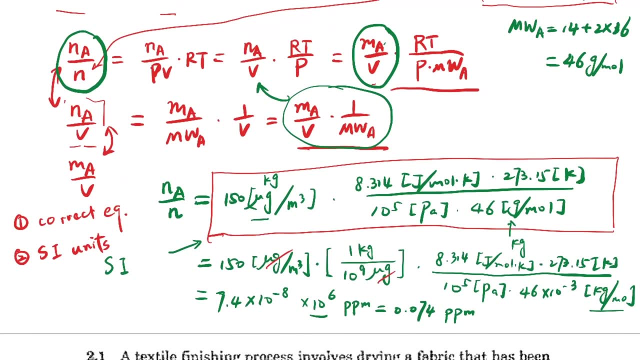 So this is a mole fraction of the solvent in the wet air. So once we know the mole fraction of the solvent in the wet air, And when we know the mole fraction, we can use this unit conversion again. right, So we can convert the mole fraction into the mass concentration. 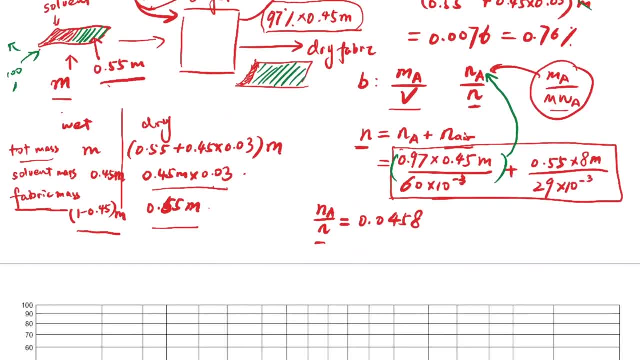 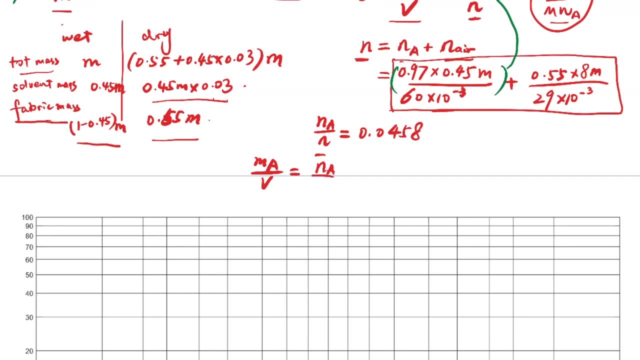 So the way we do that is basically mA divided by B is equal to mA divided by n multiplied by p, molecular weight of A divided by RT, So we have 0.0458.. Okay, multiplied by the pressure, multiplied by temperature. so I did notice, multiplied. 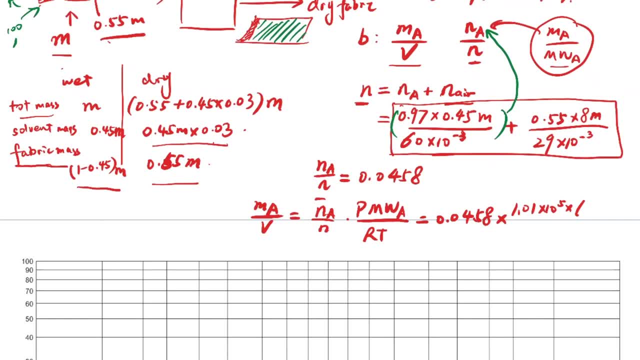 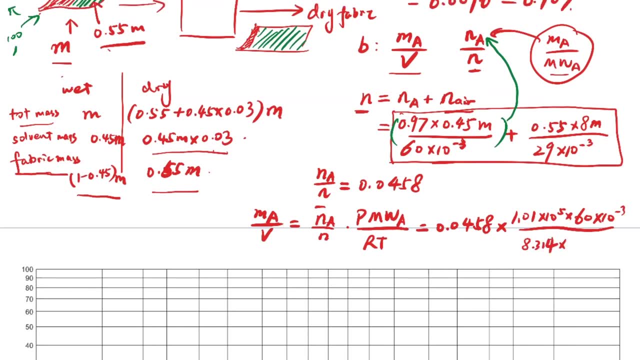 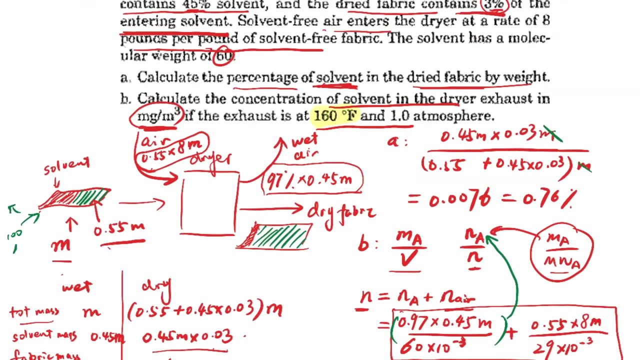 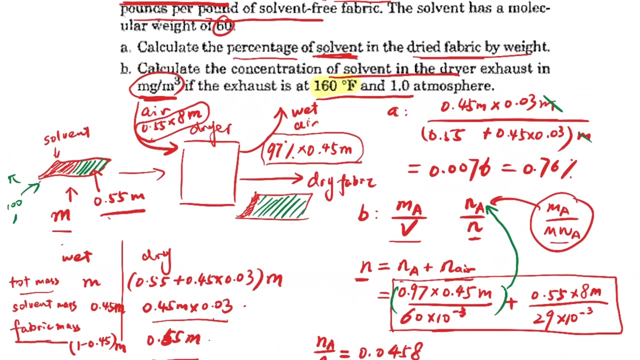 by the molecular weight, divided by 8.314 and multiplied by temperature. so I did notice that some of you actually use the directly use the Fahrenheit here, so we should use standard units, and the standard units for temperature is Kelvin, right? so you can first convert this Fahrenheit into Celsius and this is 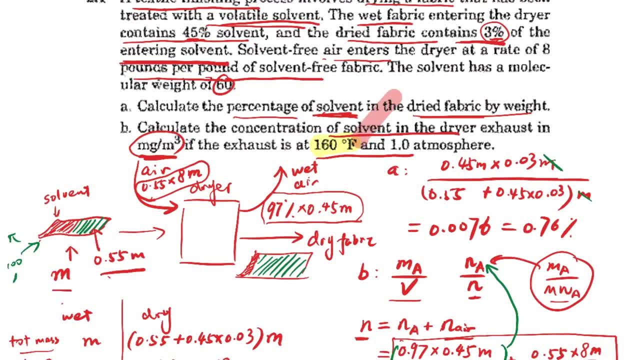 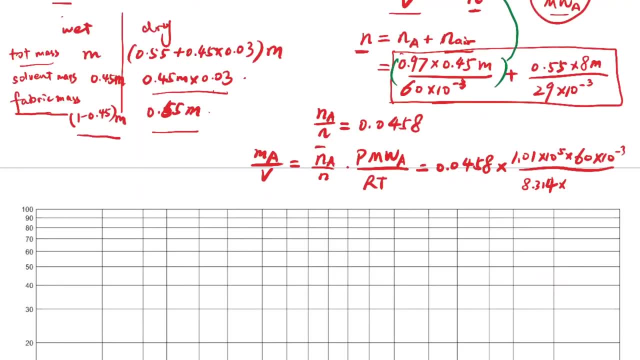 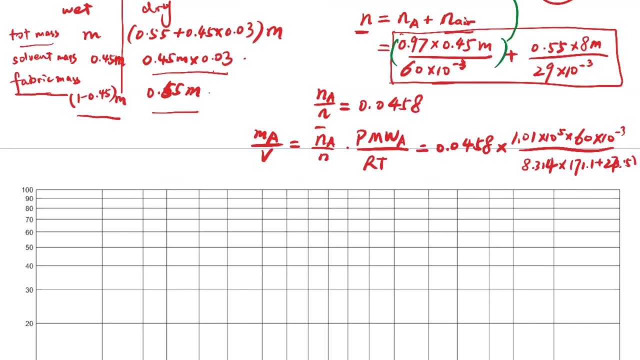 actually, and this is actually seventy one point one Celsius, right? so here, when we plug in the temperature, that will be 71.1 plus 273.15. okay, so this is the actual temperature. if you plug in this term, all of these together, you will find out that the final answer will be 0.097 kilogram per meter cubed. 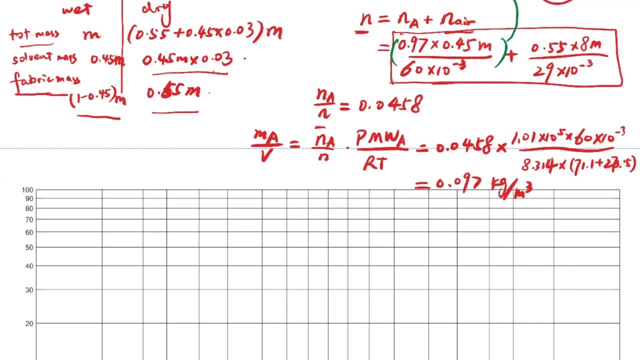 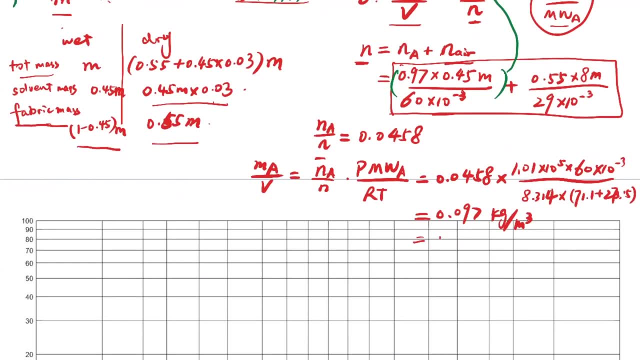 Okay. so the question asks us about the milligrams. So we need to convert the kilogram into milligrams First. we can convert that into grams per meter cube. Right a milligram. we just need to multiply that by 1000. 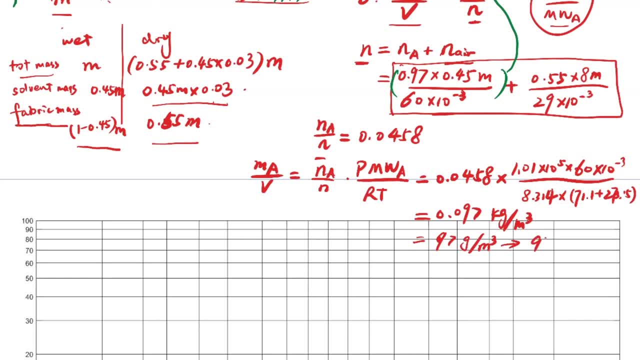 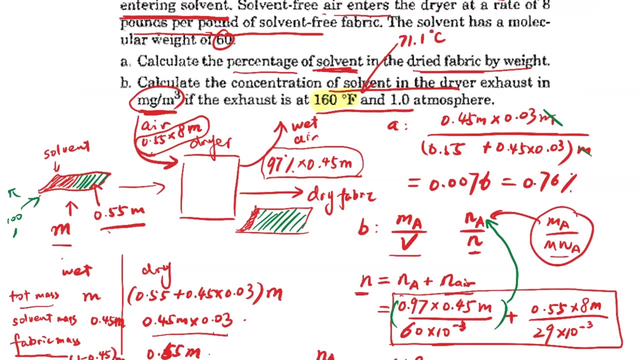 So 97,000 milligrams per meter cube. Okay, so this is the final answer. The problem might look quite complex here, But if you just notice what is the unit we're talking about and then convert that unit into some value, that is easier to solve. 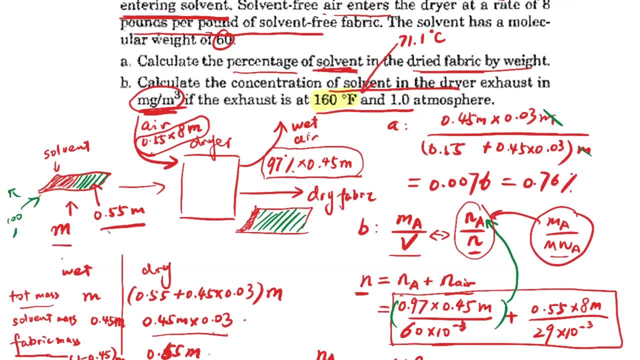 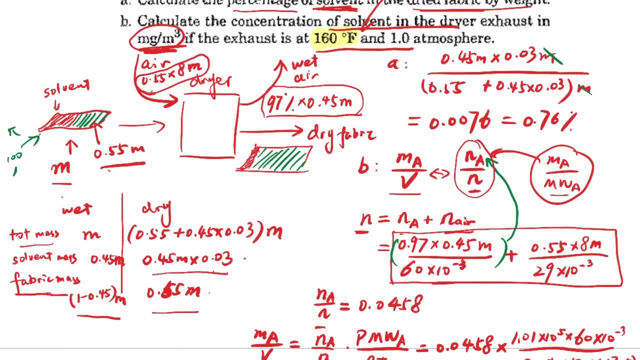 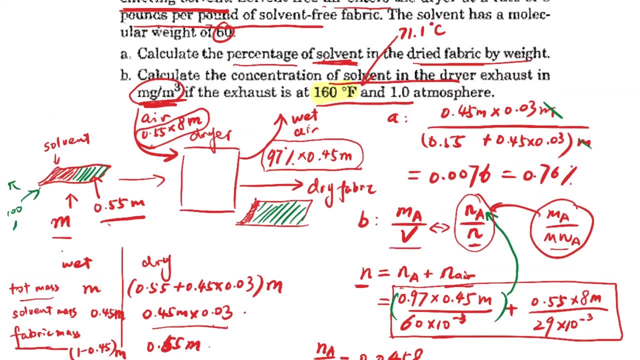 then you should be able to calculate the correct answer. Okay, So I hope that this process is clear enough. I think maybe some of you used a different method here, So here I'm just trying to relate this question into the unit conversion So it's easier to understand. 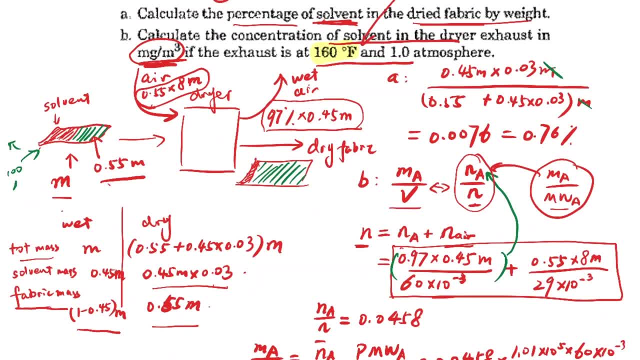 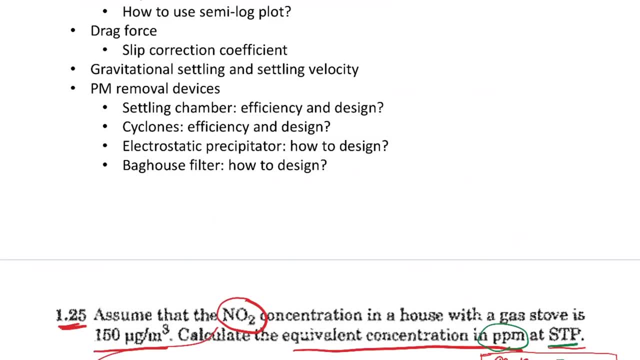 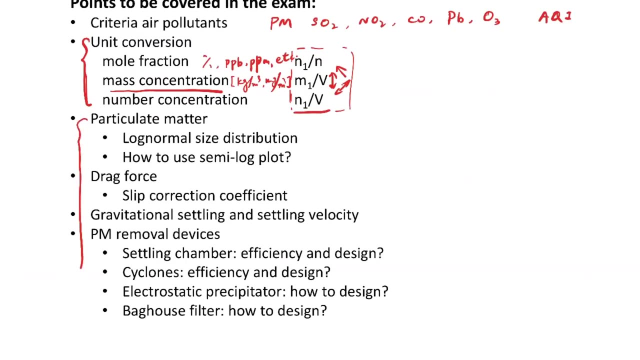 Okay, So I think for this class we just demonstrated two questions, And this is related to the unit conversion. So next class we'll go through the review contents for the PM And then we'll also go through some common problems or common questions you have in your home. 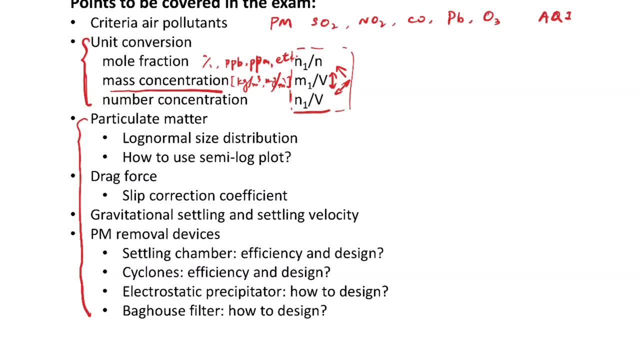 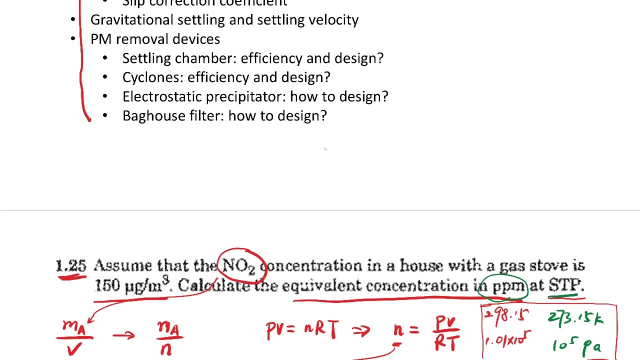 Okay, Just feel free to let me know if you have any questions. I hope that you can understand how we're doing these, how we're working these problems out Right. Can you scroll down to the answer again, please? Sure, Thank you. 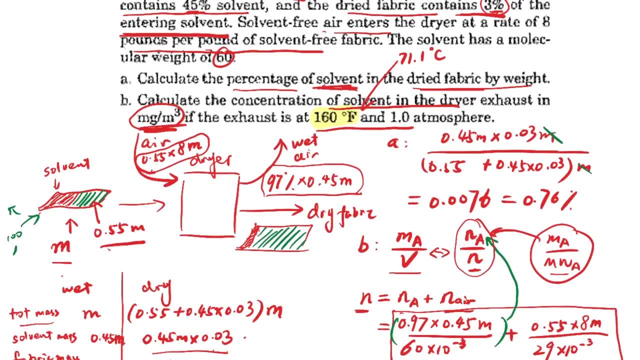 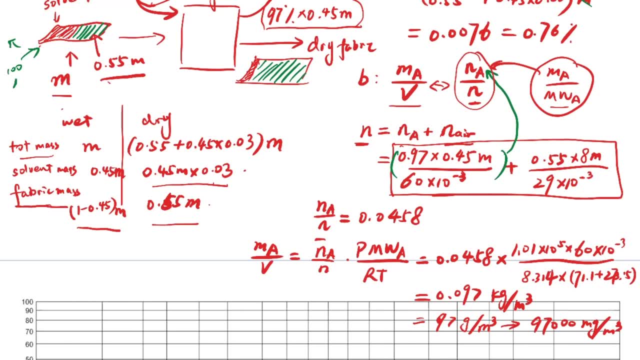 Yeah, Any other questions? Anything not clear? All right, If no more questions, I'll stay online for some longer time for you to copy the notes here, And if you don't have any other questions, feel free to leave. Okay. 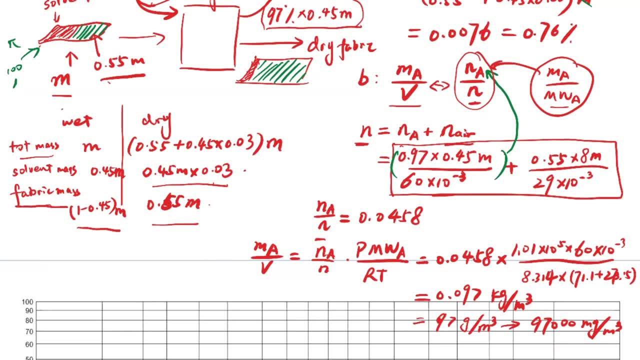 Hi Dr Ong. Yeah, So for the exams, are we going to have any questions that will require us to print out the question paper? I don't think so. Okay, So, something like the. So, for example, if we have the log, normal graph, 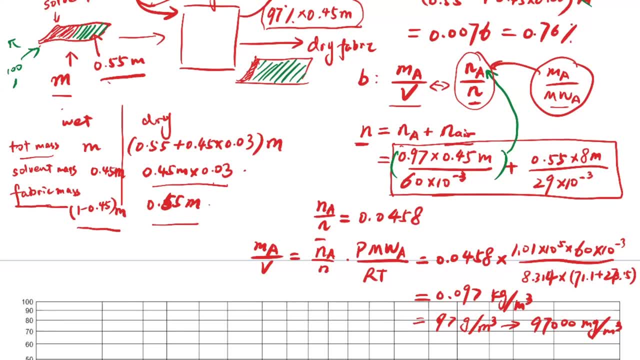 we will have to print it out and draw the curves on the graph. So if there was something like that, then I can make arrangements for printing the question and something like that. Yeah, So for those questions I was thinking you can use your previous homework sheets. 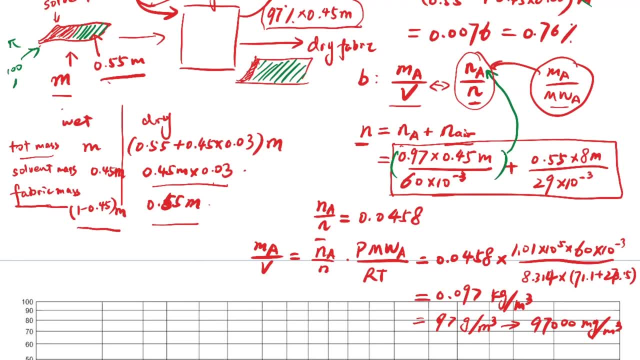 So if you still have them, Okay, Yeah, So that's a good point. I'll probably I'll send a notification on Catalyst. All right, Thanks. Or you guys can. I'll just send you a clean. I'll send you a clean piece of paper.